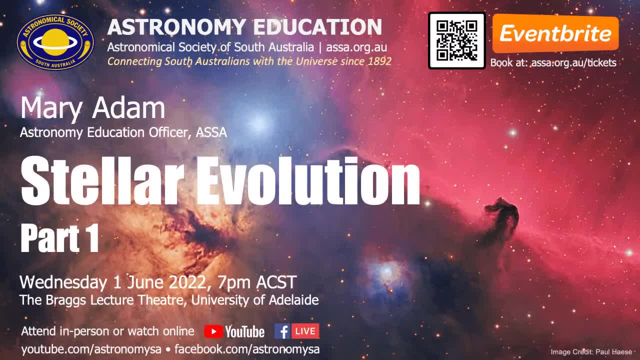 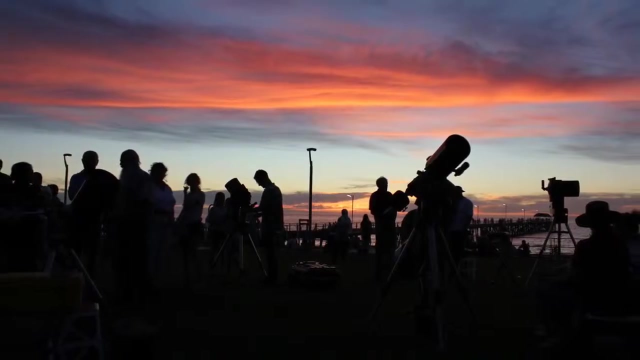 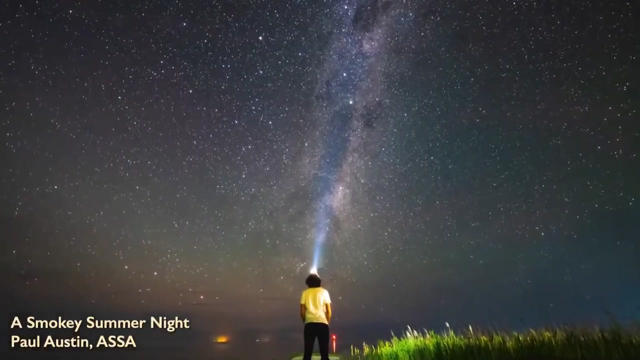 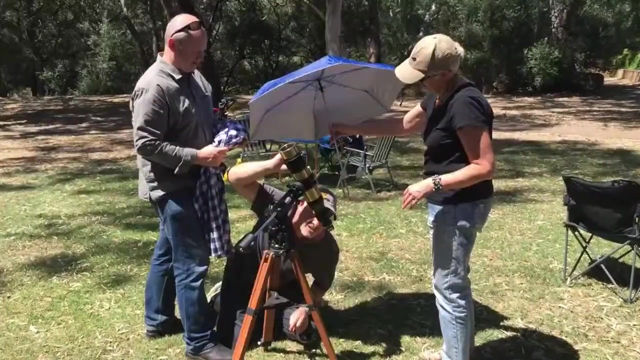 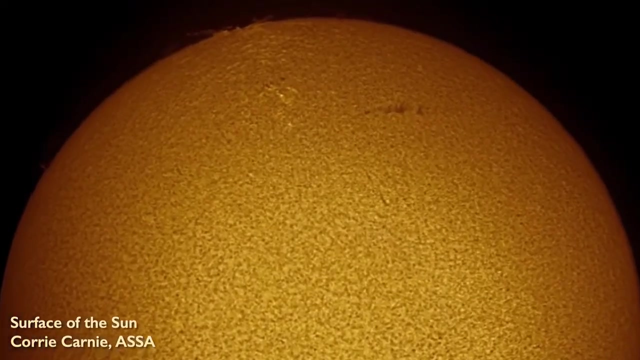 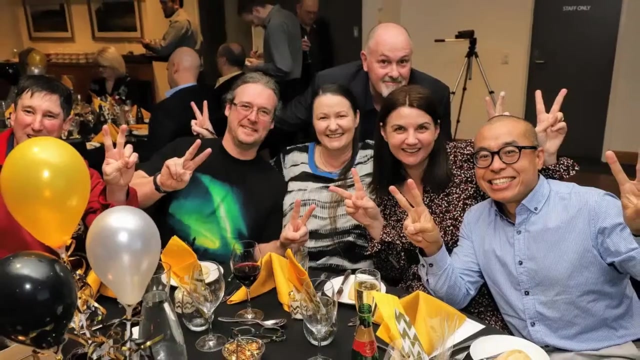 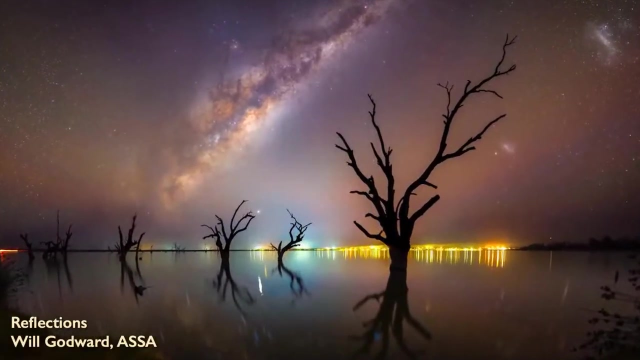 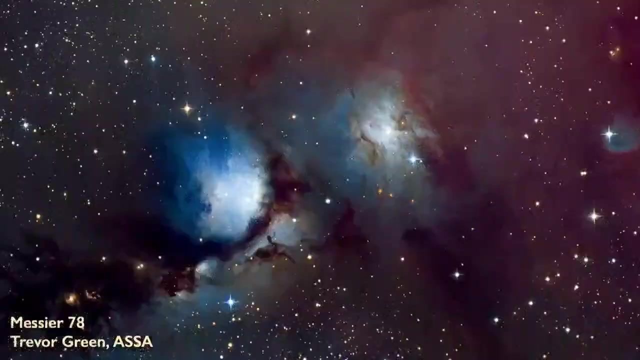 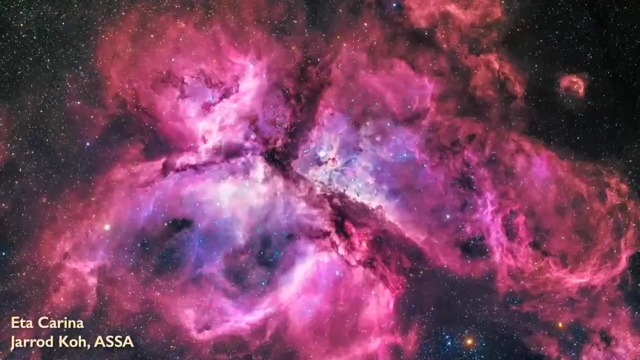 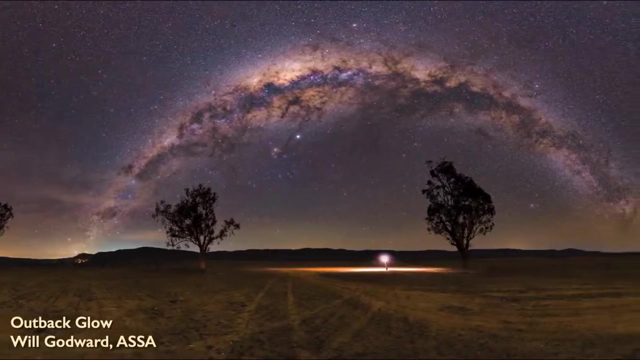 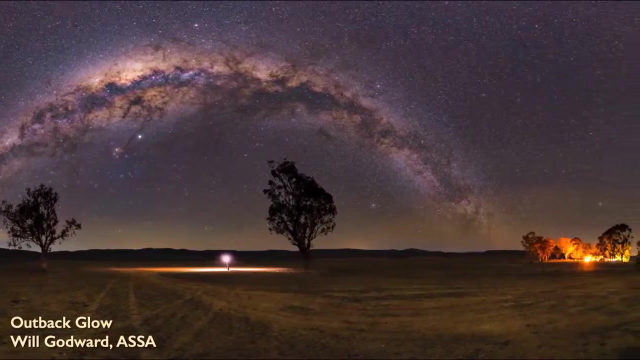 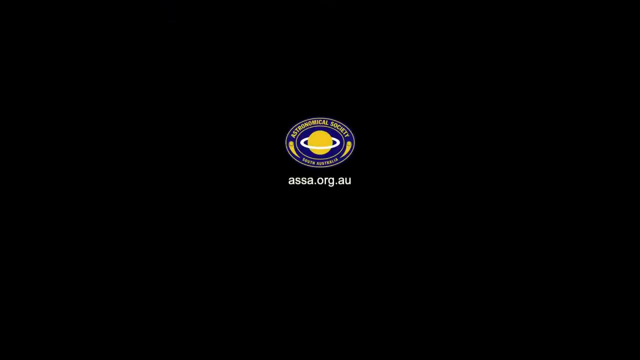 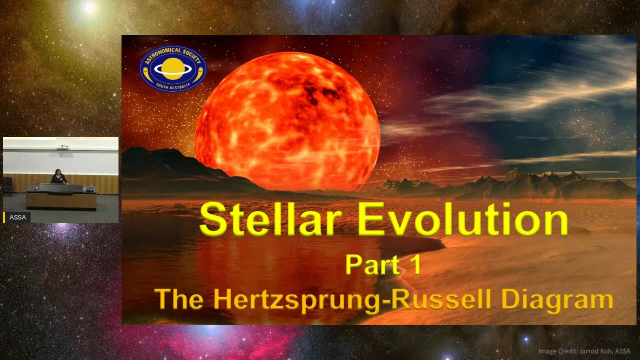 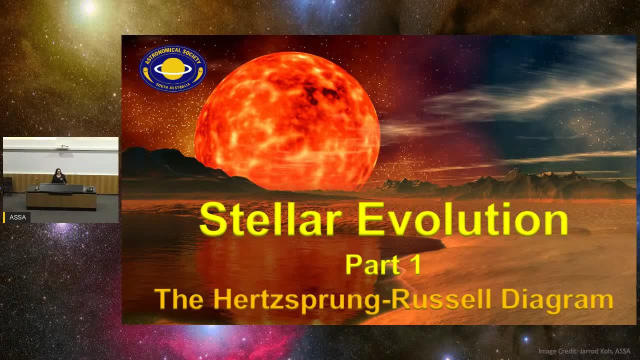 of the Adelaide Plains that we're gathered on. I acknowledge the deep and spiritual relationship the Kaurna people have to country and pay my respects to the elders past, present and emerging. Welcome to astronomy education. Today's lesson is on stellar evolution, and there's two parts to this. 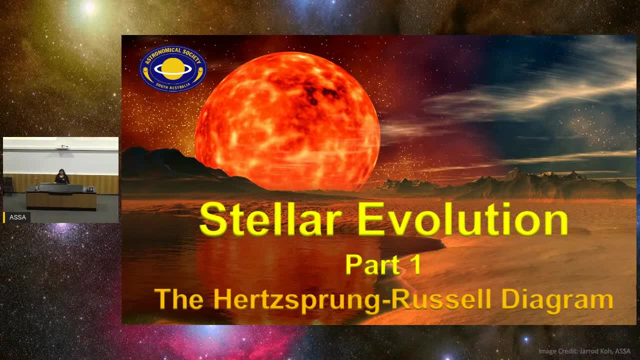 So we're going to begin with part one. The Hertzsprung-Russell diagram is where we're going to start. Just confirm me. You can all hear me up there still. Excellent, Okay, Let's do this. Stellar evolution. 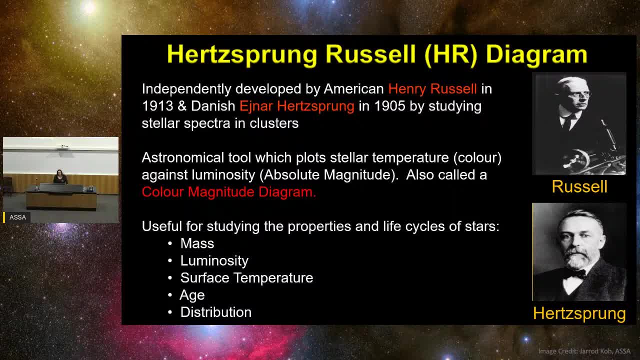 So the Hertzsprung-Russell, what we know to be as the HR diagram in astronomy, was independently developed by American Henry Russell in 1913 and Enya Hertzsprung in 1905, by studying stellar spectra in clusters. 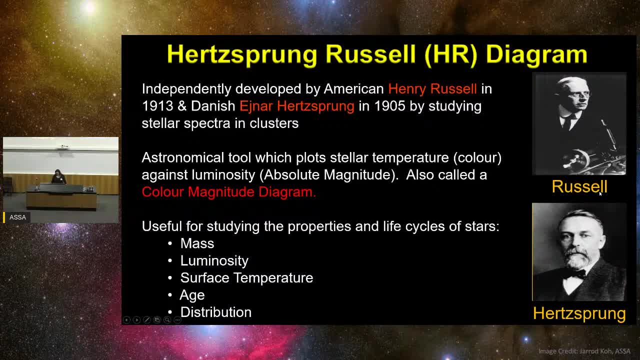 And this is Henry Russell over here and Enya Hertzsprung down here. So this is the astronomical tool we use which plots stellar temperature. When we talk about stellar temperature of stars, we're referring to their outsides and, indirectly, to the 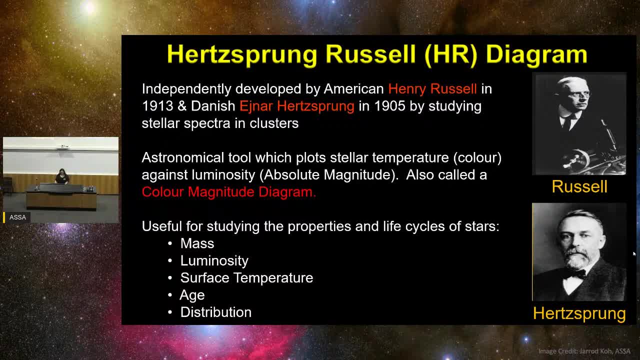 color. It's reflected in the color of the stars against luminosity, which is what. So you can think of luminosity as the energy output of a star, How it's added to the energy output of a star, So you can think of luminosity as the energy output of a star. 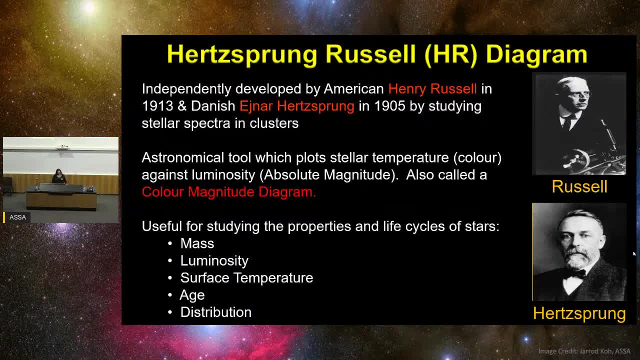 How it's added to the energy output of a star- Absolute magnitude, And this is also called a color magnitude diagram. It is useful for studying the properties and life cycles of stars, And what we use it for is to look at the mass of a star, how massive a star is. 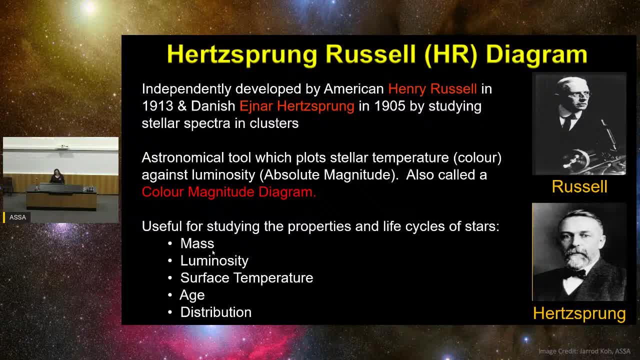 And, by the way, we compare everything to our sun. So you often see it written as a solar mass or M, with a little dot inside of a circle. So we compare it all to our sun, which is one solar mass. Luminosity again. think of luminosity as almost like the energy output that a star has. 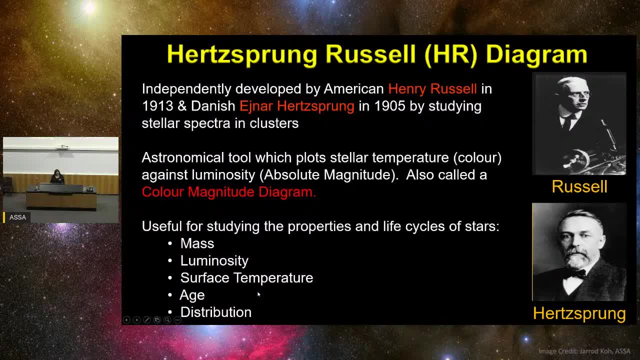 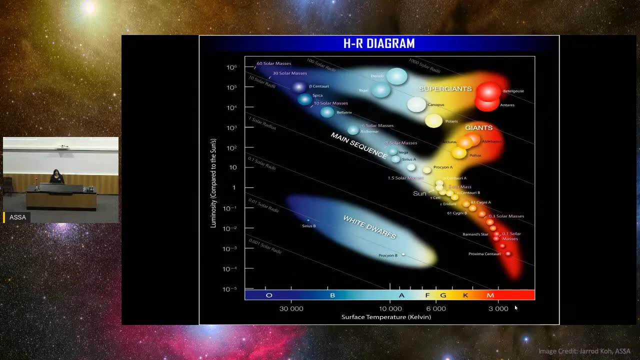 Surface temperature. again, these are all related: Age of a star and also the distribution within star clusters, And this is what it looks like. So the main part will first grab you is this part here. This is what we call- and I'm using the mouse, by the way, because there's people online- 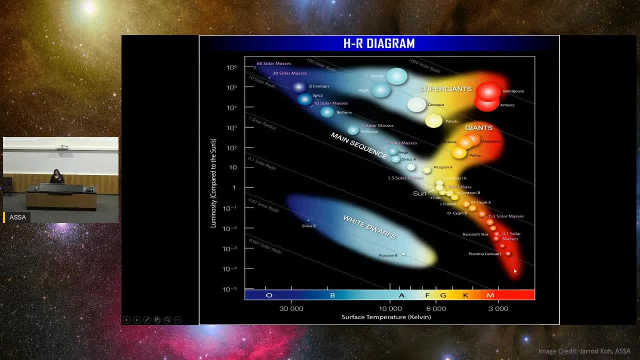 who won't be able to see the pointer, But this is what we call the main sequence line through here. Now, a main sequence star is basically a star burning hydrogen. The first phase of a star's life, once it ignites, is its hydrogen burning stage, where 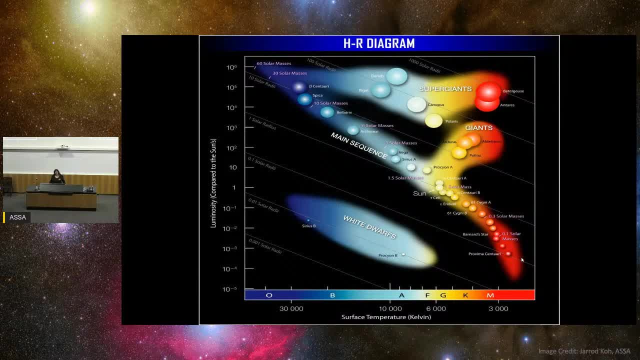 it's fusing hydrogen into helium And all the stars along this particular path. Here are what we call main sequence stars. We also call them dwarfs. regardless of how big some of these stars might be, We refer to this particular grouping as dwarfs again because they're on their first stage. 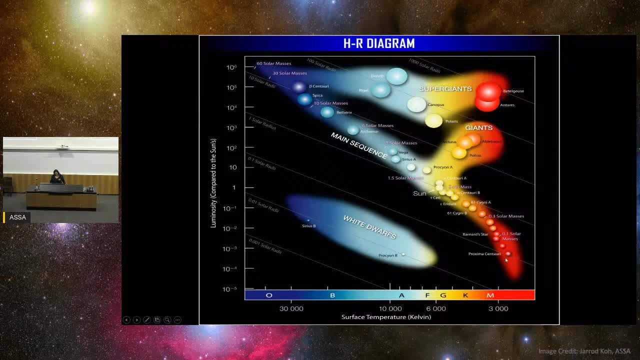 So if you look right down here in the red we have Proxima Centauri, the closest star system to our sun, about 4.2 light years away. It's a red dwarf, Bernard, star down here, 1 tenth. 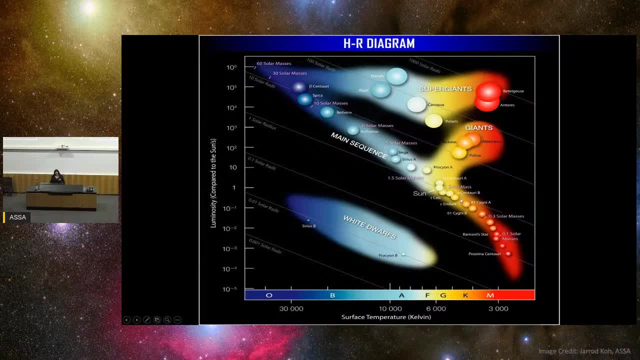 1 tenth. That's the mass of our sun And our sun sitting over here, a G25 yellow dwarf Off to one side you'll notice there are giants. Now this is where our sun's going to start moving off into once it comes off the main. 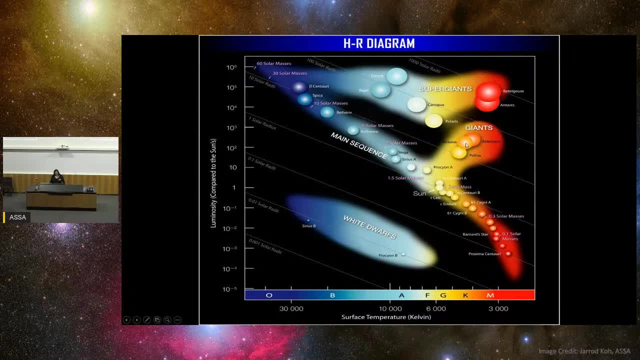 sequence. And there's the notable stars Arcturus, Aldebaran, Pollux- These are stars that are in their giant phase- Sirius A and Vega- again, the three solar masses around here. they all still sit on the same, on that main sequence. 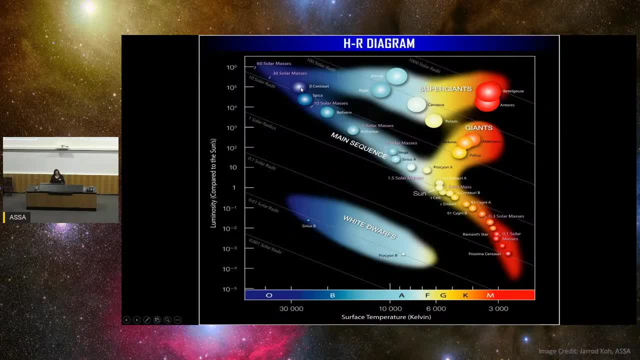 Achenar, Bellatrix, Hadar, the star, Beta, Centauri, up here now. they all look so different to us. Their colours are so different because of their temperatures, but they are all still in their main sequence phase: burning hydrogen into helium. 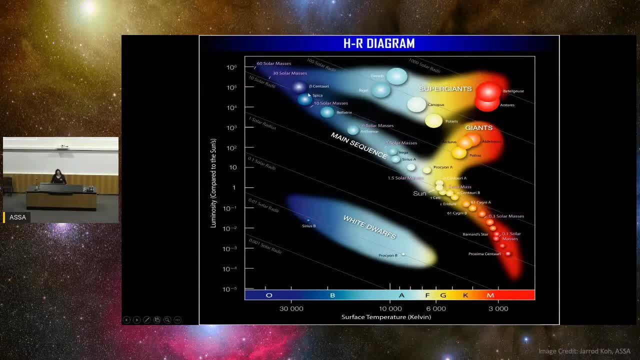 Massive stars that come up to here, around 30 solar masses. you know, even down here 10 to 15 solar masses will move off Once they come off the main sequence. they're still in their giant phase Once they come off the main sequence and they're no longer in their hydrogen-burning 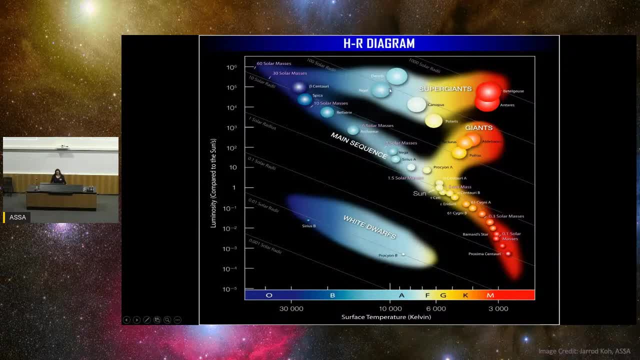 phase they move into what we call supergiants, And this is where you'll find Rigel Deneb, the tail of the Swan, in Cygnus, Canopus in the constellation of Carina, the second brightest star, and, of course, Betelgeuse and Antares. 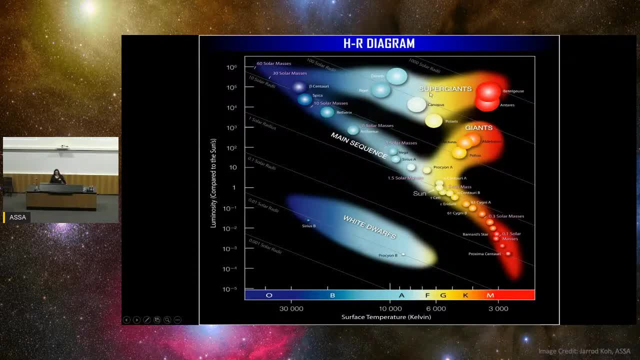 the red supergiant. So these stars are not what we call main sequence stars. These are supergiants Down here we have white dwarfs. Now if we look at the colour of these particular stars, Sirius B: extremely hot, almost 30,000. 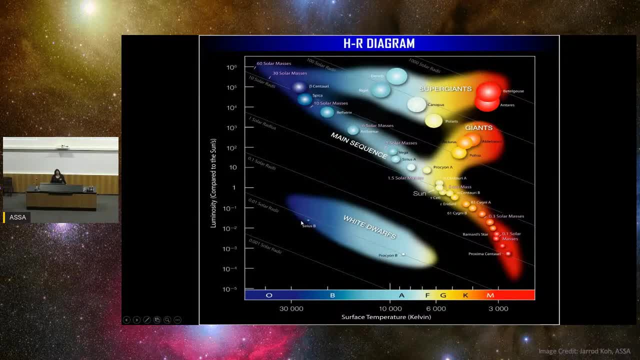 Kelvins, but very, very dim, because they're not very big at all. they're quite small. Same here with Procyon B, much, much hotter than the surface of our Sun, but a lot fainter. So this is the HR diagram. 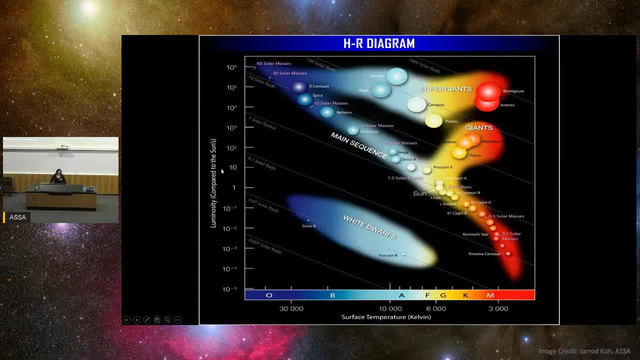 So over here on the right- sorry, on this side- you have luminosity again. compared to the Sun's luminosity, It's one one. our Sun sits right here at number one, so we compare everything to it. So stars much, much more luminous than our Sun, up to a million times more luminous, right. 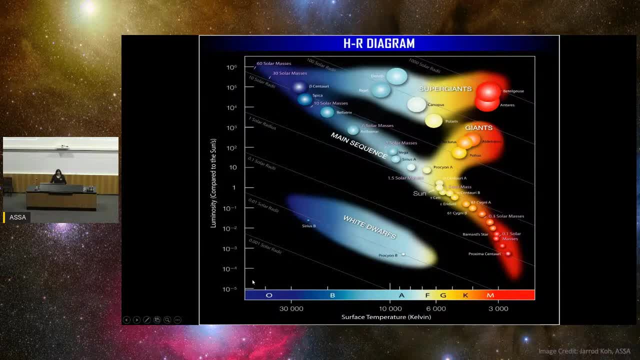 the way down to the dwarfs down here, And also if you look at Proxima Centauri and come across nowhere near as luminous as our Sun, And down here is the surface temperature in Kelvins of the outside of a star. 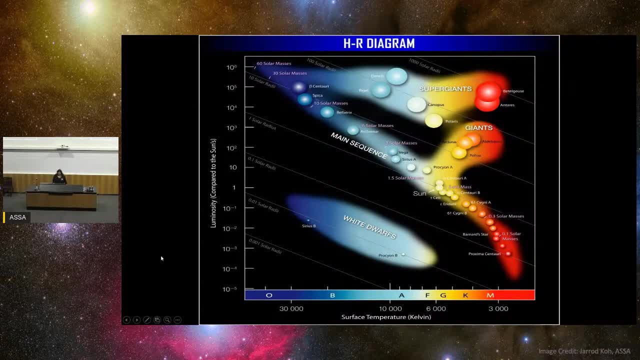 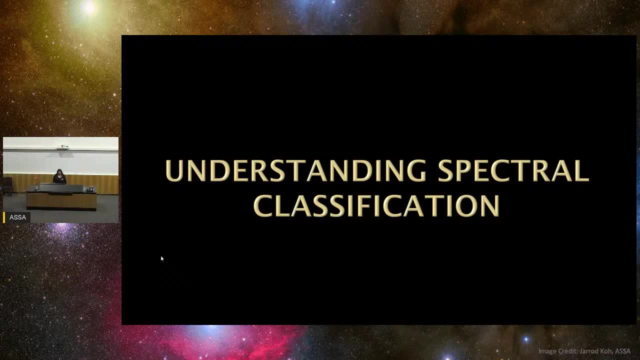 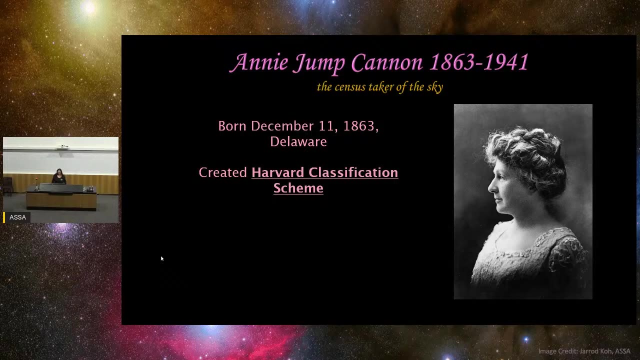 The surface temperature. Now to understand a spectral classification a little bit further, I'm going to introduce you to two amazing women. This one here is Annie Jump Cannon, born in 1863. She's known as the census taker of the sky. 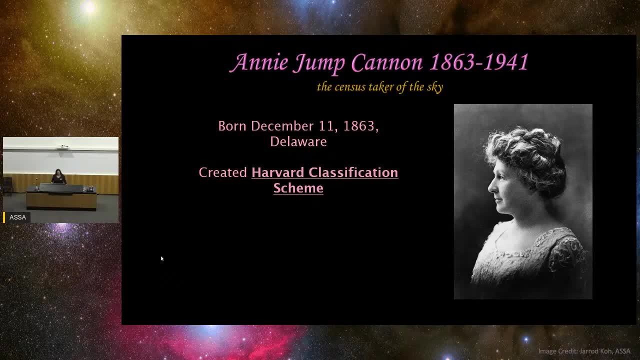 Born in 1863 in Delaware, she created what we know to be the Harvard Classification Scheme, And this was to organize and classify the stars based on their temporal temperatures and spectral types- Mainly their spectral types, though, so this is what she spent her time doing. 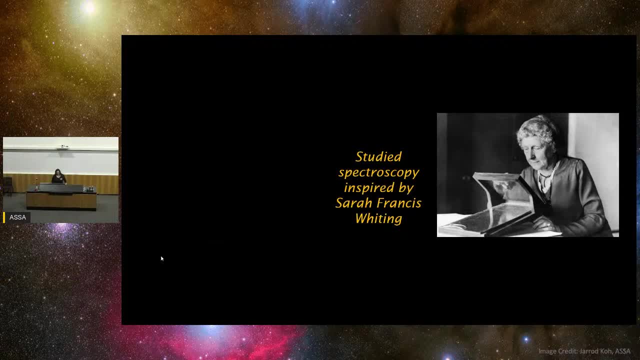 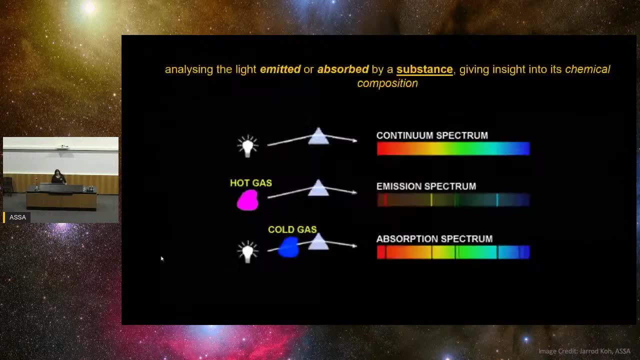 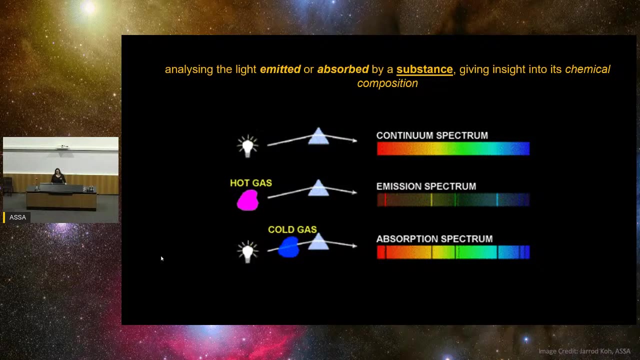 So here she is. in her later years She studied spectroscopy inspired by this, another brilliant woman, Sarah Frances Whiting. So spectroscopy is analyzing light that is either emitted or absorbed, Or, if it's absorbed by a substance, giving insight into its chemical composition. 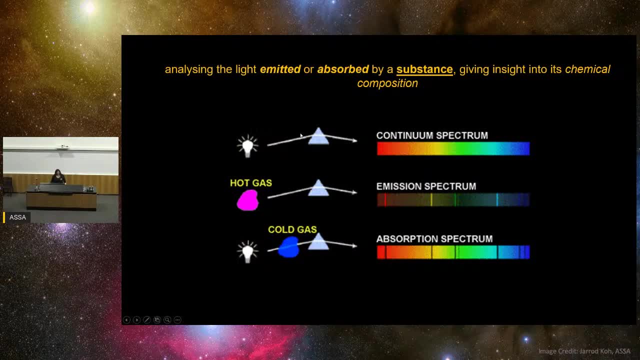 So when we look over here, we have a bulb, a light bulb over here. Put that light bulb- it's light passed through a prism and you get this continuum spectrum. If you've got a hot gas and you pass that light that's coming from that hot gas through. 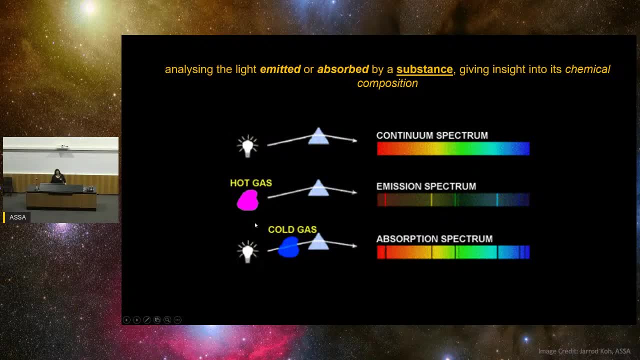 a prism, you get what we call an emission spectrum. Okay, You take light and you pass it through a cold gas, for example our atmosphere, and split that through a prism. you get what we call the absorption spectrum. So this matches those lines there. 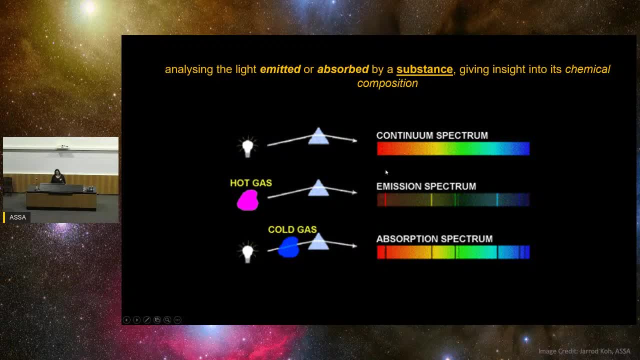 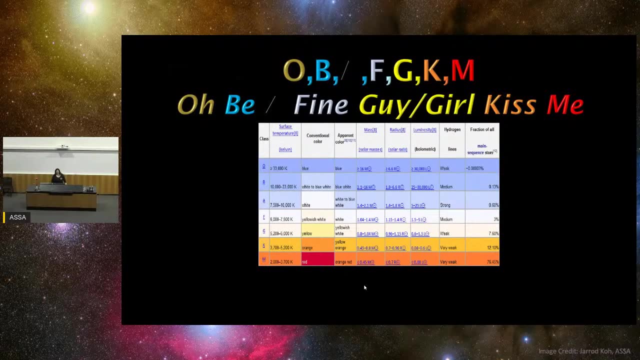 So this is an absorption spectrum and an emission spectrum and a continuum spectrum. So her classification scheme is this: that she created OBFGKM or OB. a fine guy or girl kiss me. This is how we learn this particular order of classification. So O class stars up here. they are the hottest, the surface temperature above 33,000 Kelvins. 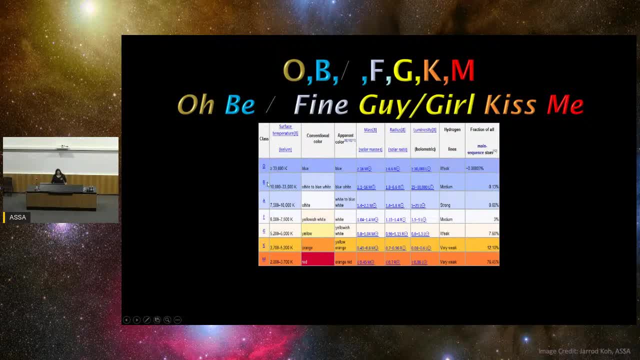 And they do. they appear blue because they're very, very hot And you come all the way down BAEFG. Our sun sits here between 5,200 Kelvins to 6,000 Kelvin. Our sun sits at about 5,700 Kelvins. 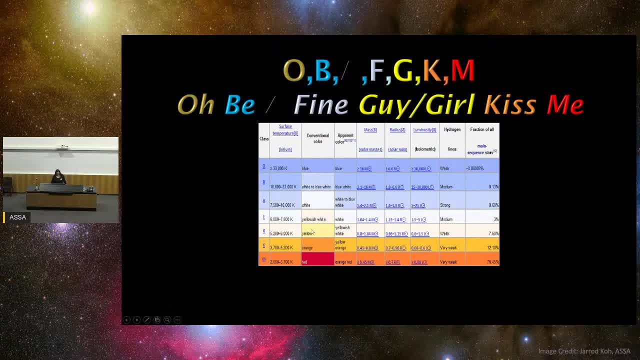 And it actually appears yellow because, again, of its color. And if you look at the hydrogen lines, this is really interesting, very weak hydrogen lines. Right the way down to your M class stars, which are your red dwarfs, They appear orange, red. 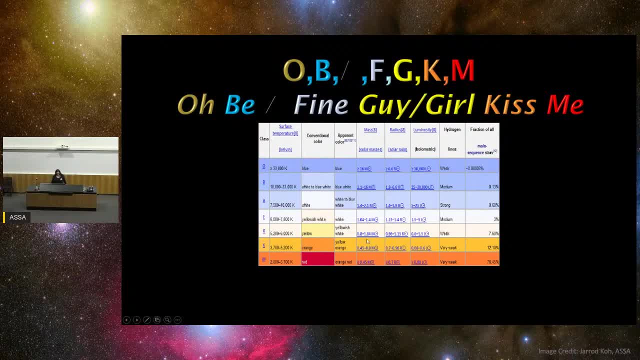 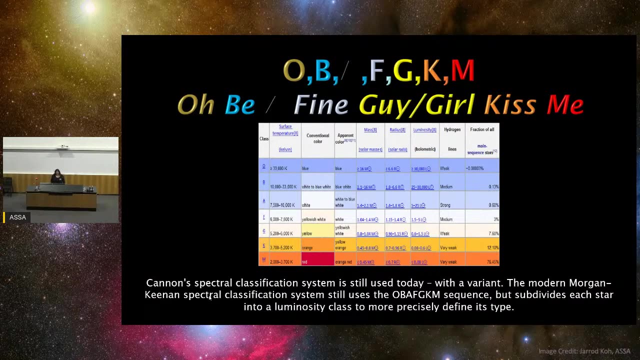 And again, if you look at the solar map, The masses, they actually start to decrease. So your more massive stars are much hotter. So her Canon Spectral Classification System is still used today, but with a variant. So the modern Morgan Keenan Spectral Classification System still uses this OBAFGKM sequence, but 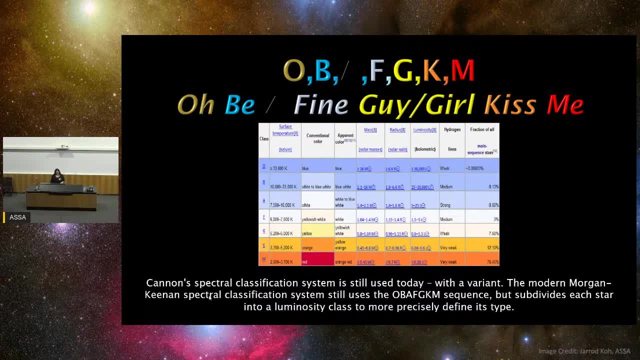 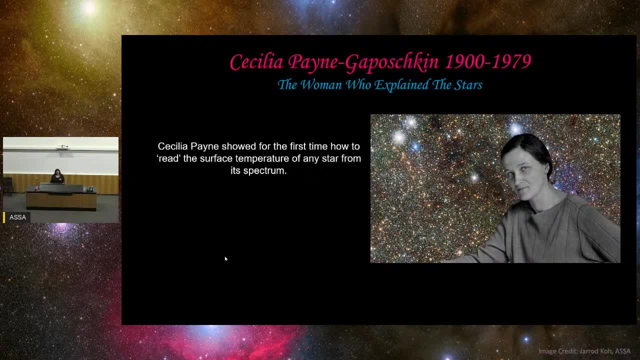 it subdivides each star into a luminosity class to more precisely define itself. Now, this is the other woman who has. I think we all should know about, Cecilia Payne Kaposchkin. This is the woman who explained the stars. 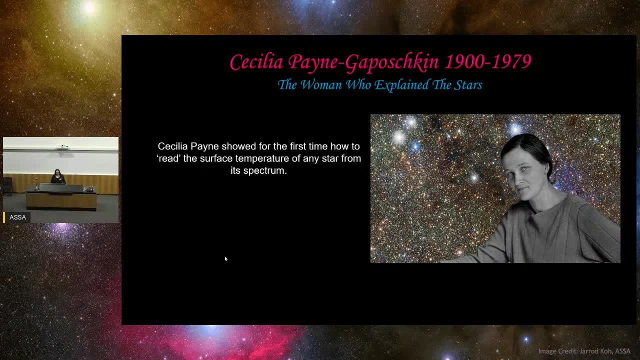 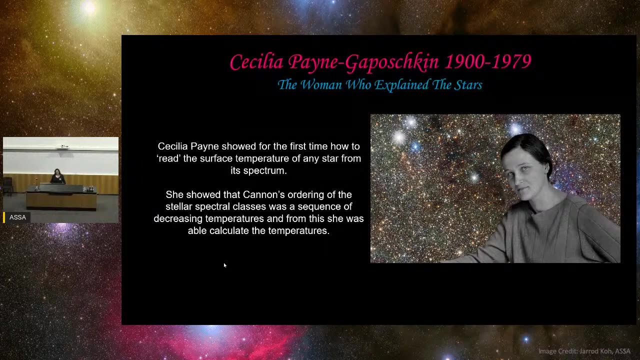 And she showed for the first time how to read the surface temperature of any star from its spectrum. And she showed that Canon's ordering of the stellar spectral classes was a sequence of decreasing temperature And from this She was also able to calculate temperatures of the stars. 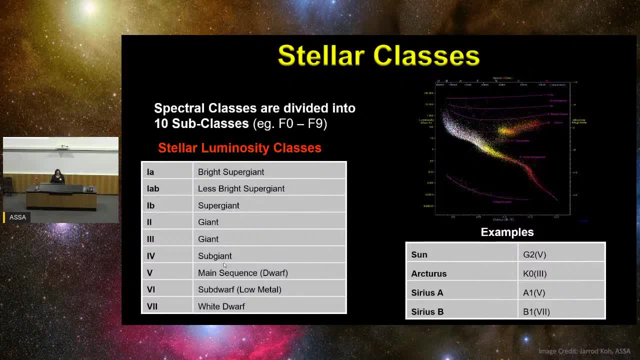 So another incredible woman. So the stellar classes. if we look at them, the spectral classes divided into 10 subclasses. Example: with your F class stars, they go from F0 to F9. So this is what we talk about when we say stellar luminosity classes. 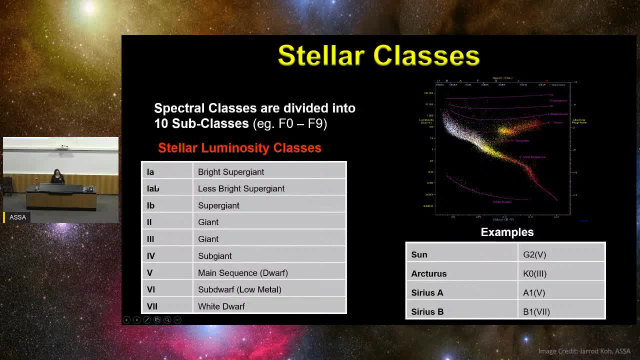 One A is a bright supergiant, One AB a less bright supergiant, And then and so on, Your supergiants, your giants, your subgiants, your main sequence dwarf like our sun, right down to your white dwarf. 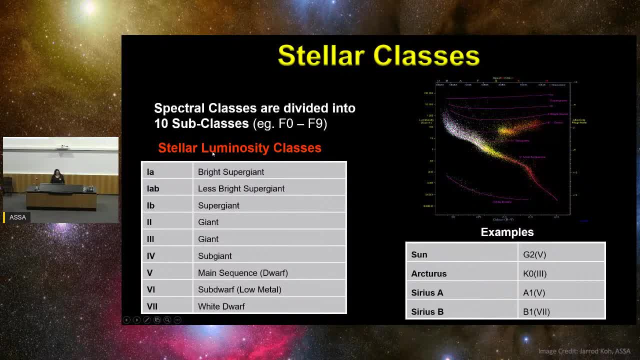 So it categorizes them based on their luminosity. So excellent examples: over here, Our sun, a G2 star, G25.. So there's your color index down here, And our sun sits around. Where are we Around here? Arcturus, which is a K03.. 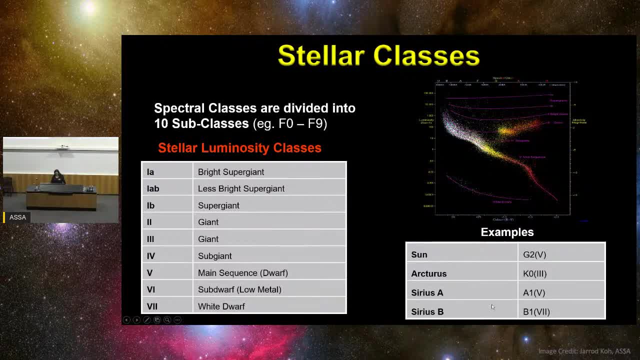 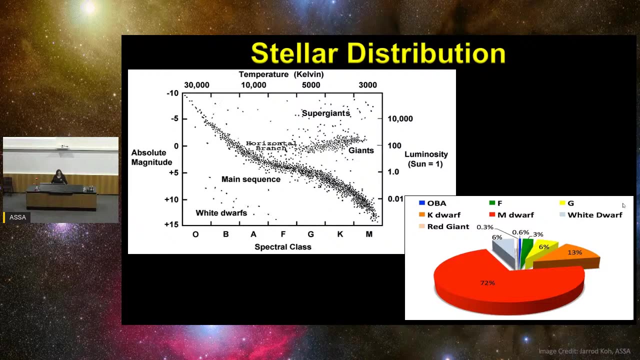 Sirius A, it's an A15.. And Sirius B, a B17.. So this is how we break them down even further by their luminosity, And so what's interesting is also the pattern of stellar distribution among these within this diagram. 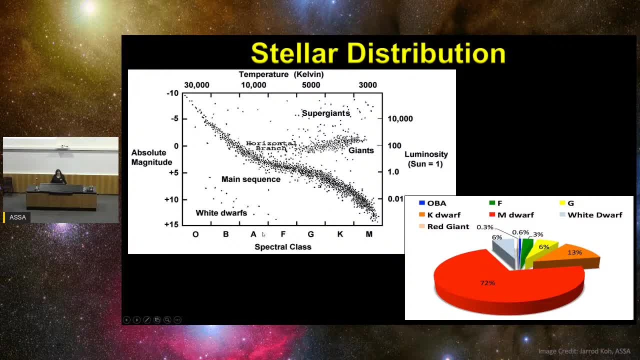 So here you have your spectral class, your main sequence, again along here, What we call the horizontal branch. here your giants, your supergiants, your white dwarfs, This is where you'll find them. So OBA stars make up just a tiny amount: 0.6% of stars that we see. 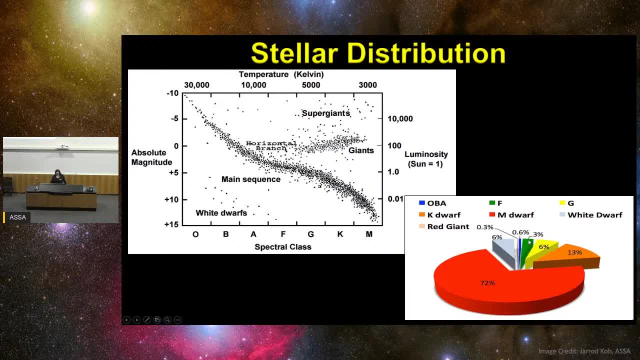 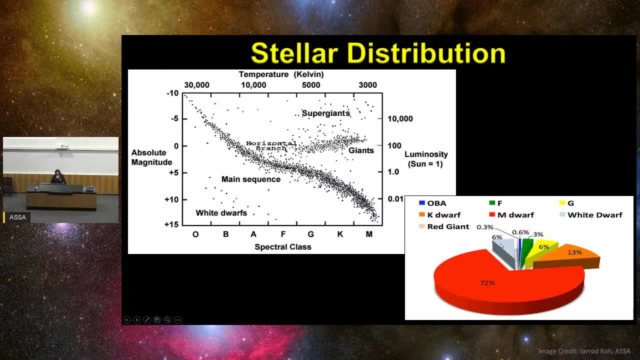 And then you've got your G stars, like our sun white dwarfs- again about 6%, Your K orange stars, your K dwarfs down here, 13%. And what's really interesting here is the M dwarfs. your red dwarfs are the most common. 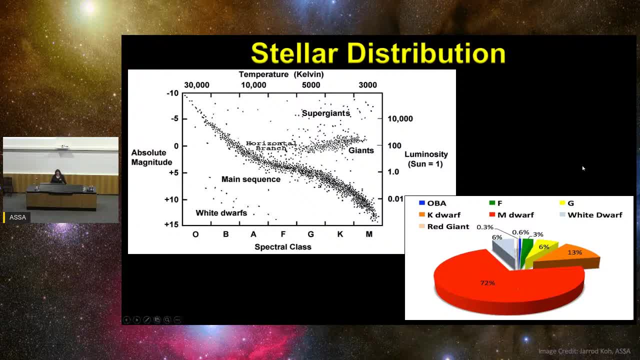 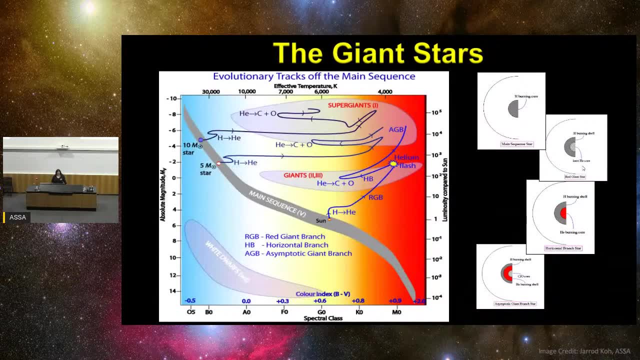 types of stars in the universe. Um, Uh, Um. So if we look at the giant stars, this is a great diagram. this one here, this evolutionary, tracks off the main sequence. So again, here we have our Sun sitting at number 1.. 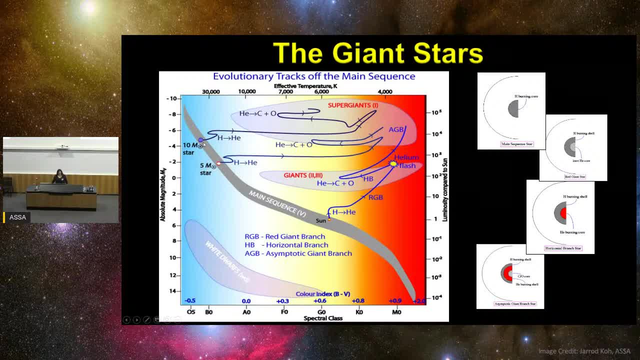 Here we have a star, a 5 solar mass star, a 10 solar mass star. so as we have a look at our Sun here as it starts to run out of once it starts well, here we have it actually burning hydrogen into helium, but that actually will eventually run out. 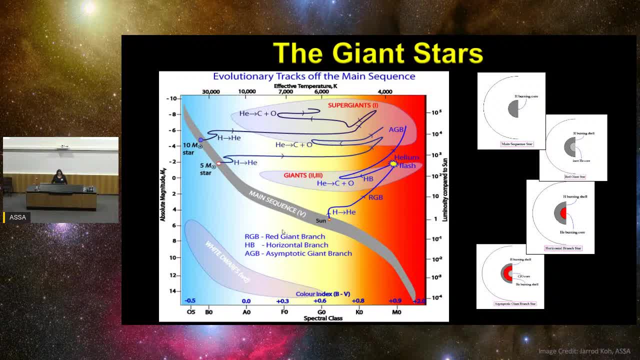 The fuel in the centre will expire. where's my mouse? here we go, and as it does this, it becomes what we call a red giant. it's going to start fusing its helium once it runs out of hydrogen. the Sun's core is actually going to get much, much hotter. 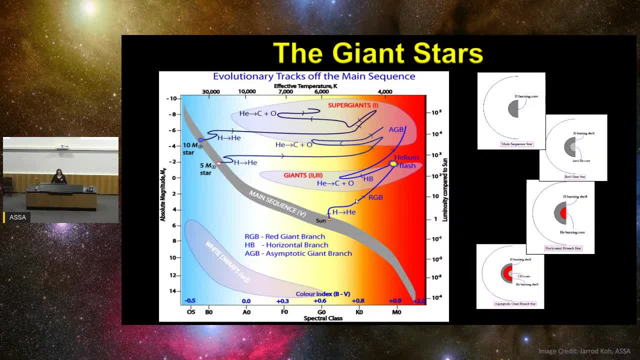 It's actually gravity that does this. it tries to. it will try and crush the star as it runs out. It will, but the crushing actually saves it. it drives the temperature up to about 100 million degrees, and that's the temperature needed for the helium ash in its core, the 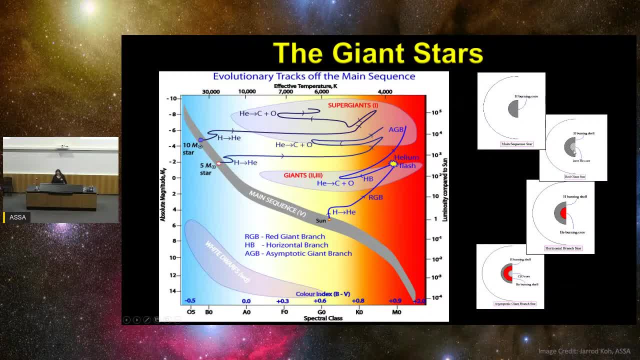 inert helium in the core over here. So you see the hydrogen burning core now in our main sequence star. it becomes a red giant when the it has an inert core hydrogen burning shell still on the outside, but the crushing actually drives the temperature up to about 100 million degrees and at that temperature 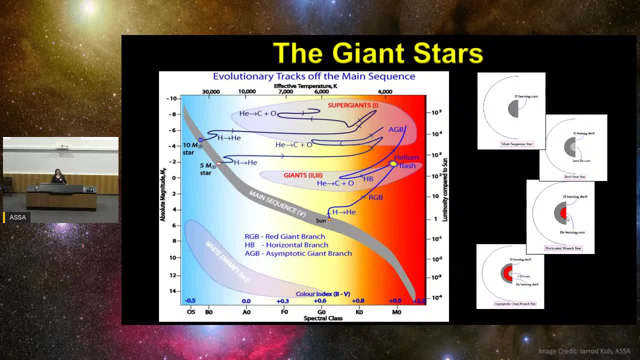 helium will start to burn, start to fuse in its core And that's why the star expands and it just swells up. you've got a lot more thermonuclear radiation pushing the star outwards. the star swells up and the surface actually cools. 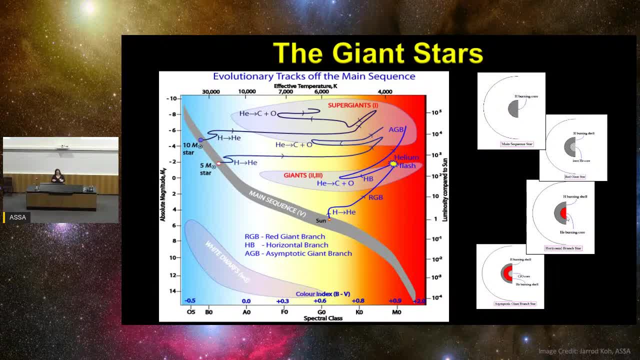 down because it's much further away now from the core. so these stars, their cores are much hotter, the surfaces are much cooler, but their cores are actually much hotter. And so this is when it moves on to our horizontal branch star over here. so it moves up and 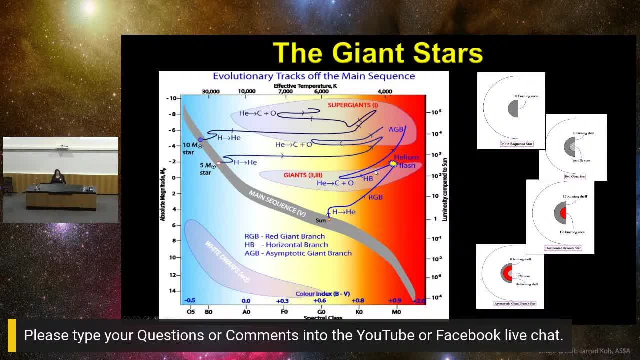 it's going to do what we call a helium flash, and then it's going to come right back down here. Now, once it starts fusing its helium, it doesn't have as much helium as it did hydrogen initially, so it's going to burn through it much faster. and once it's used up, as it's burning helium- 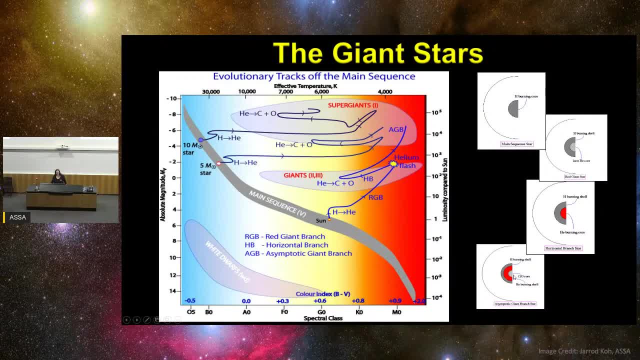 so it's going to start dumping carbon and oxygen into its core, this inert carbon and oxygen that you see down here. So once it runs out of its helium, the same thing's going to happen: gravity's going to try and crush the star again. when you crush a gas very quickly, you heat it up, shoots. 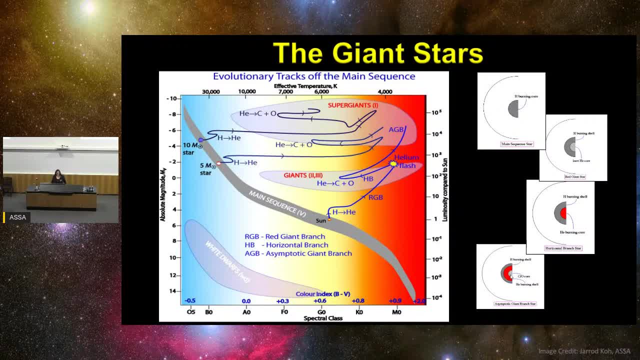 the temperature up, in this case to about 500 million degrees. that sort of temperature is what you need in order for carbon to start fusing, But our sun doesn't have enough mass to sustain that sort of fusion. and also at 500 million. 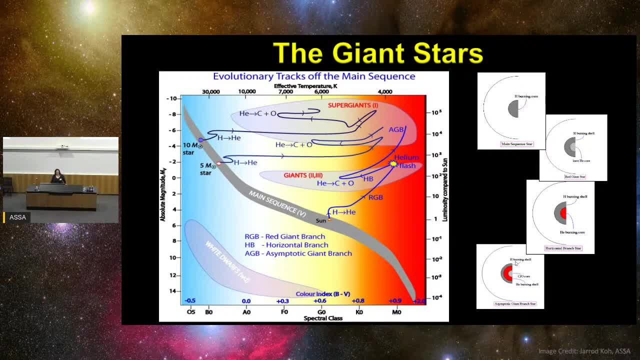 degrees, you get the star blowing right out. It's actually going to go through two red giant phases and an orange giant would become a red giant, then an orange giant, then a red giant, again much, much bigger the second time around, and at 500 million degrees pushing outwards, the surface actually just slips. 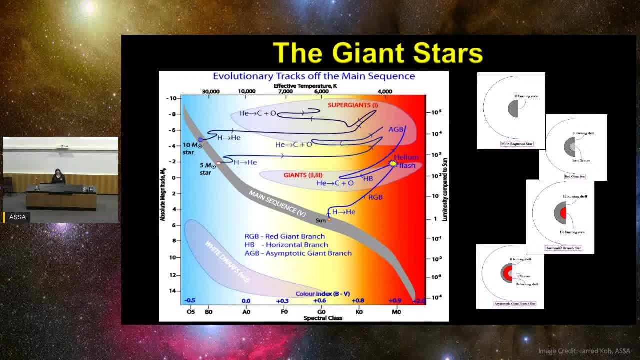 away, puffs away and becomes what we know as a planetary nebula. So our star's not going to go bang. only big stars go bang. our star won't. but this is the life cycle here for our star, where it will eventually end up. what's left will be. 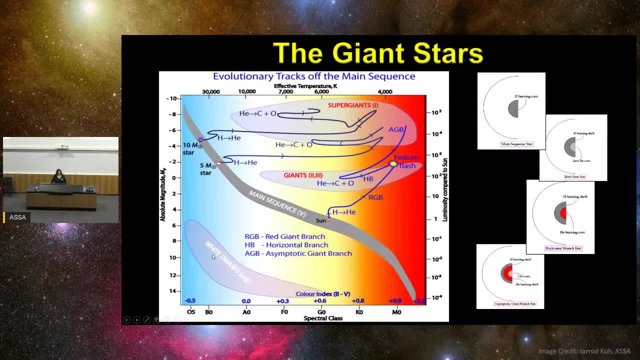 about the size of the Earth. the core will end up as a white dwarf, So very, very hot remnant sitting way down here, sorry. So very hot, but not as luminous because it's obviously not going to be as big. 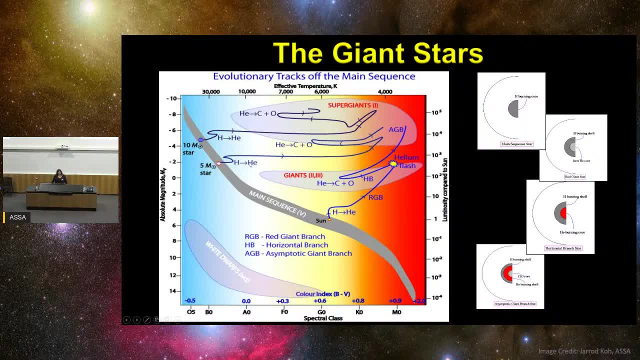 A star with five times the mass of the sun. same thing: hydrogen fuses into helium. it's going to move. It's going to move along up here, move into its carbon and oxygen burning and end up over here, your 10-mass star. this is where it starts to get interesting. 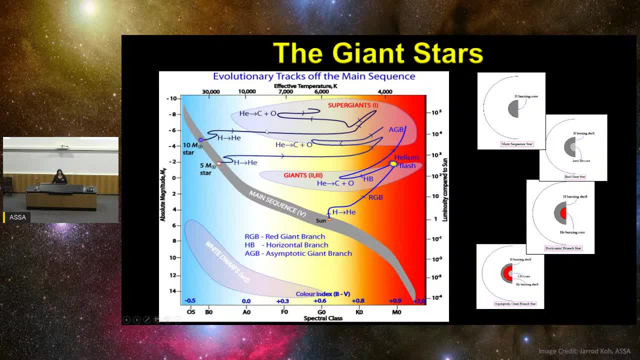 It will do the same thing: use up its fuel of hydrogen, start burning helium. it can sustain helium, carbon and oxygen, and it just keeps going. Stars like Betelgeuse Anteros. they'll just keep burning heavier and heavier elements. 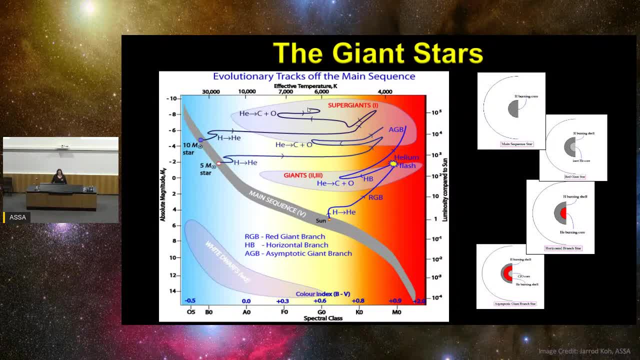 right the way up to iron. Once a star produces iron, within a day it's dead. Iron doesn't free energy, it doesn't liberate it, it absorbs it. So this is the evolutionary tracks off the main sequence. so again, different for depending. 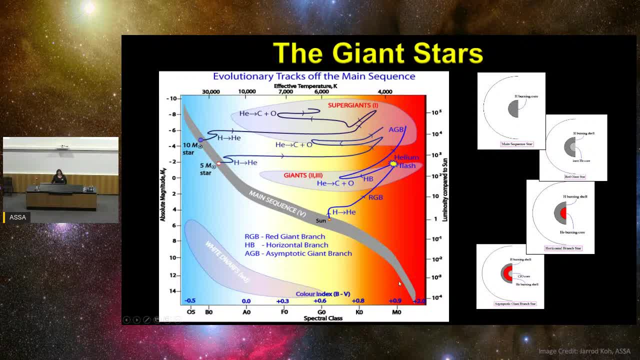 on how massive the star is. to start with, It's interesting. we can't show you anything down here. The red dwarfs: we've never seen one die, So we think because of the way they fuse their energy they burn a little bit differently. 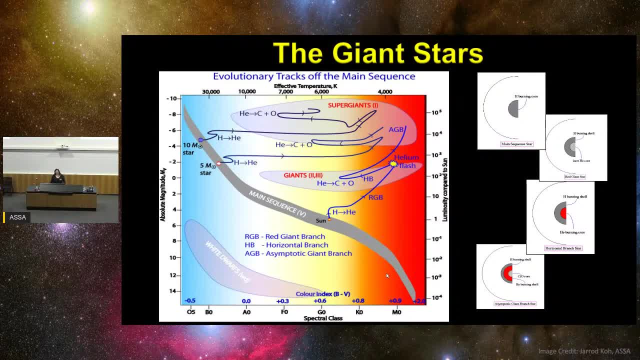 that the universe just isn't old enough. We haven't seen a red dwarf die. We think they'll go for trillions of years. So your red giant here, your RGB, your red giant branch over here, your horizontal branch here and your asymptote giant branch up here. 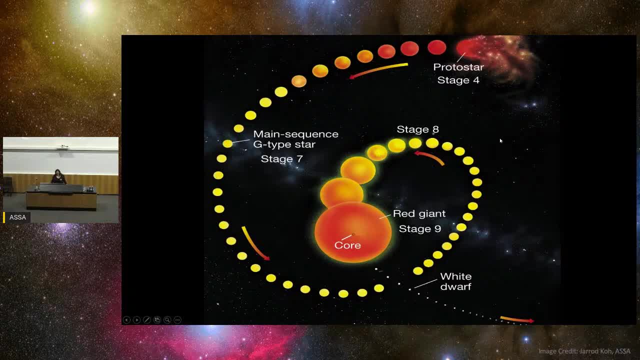 Next one. So 8., 5., 6., 7., 8., 9., 10., 11., 11., 12., 13., 14., 15., 16., 17. 18.. 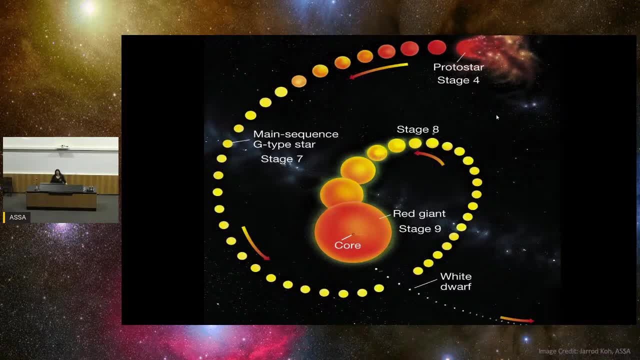 19., 20., 21., 22., 23., 24., 25., 26., 27., 28., 29., 30., 31., 32., 33., 34., 35.. 36., 36., 37., 37., 38., 38., 39., 39., 40., 41., 41., 42., 42., 43., 44., 44., 45.. 46., 46., 47., 48., 49., 49., 50., 51., 52., 52., 53., 54., 55., 56., 57., 58., 59.. 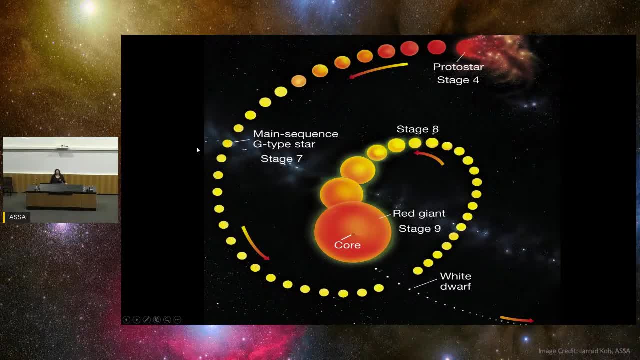 60., 61., 62., 62., 63., 63., 64., 65., 66., 67., 68., 67., 68., 69., 69., 70., 71.. 72., 72., 73., 74., 74., 75., 75., 76., 77., 78., 78., 79., 79., 80., 80., 81., 81.. 82., 82., 83., 83., 84., 84., 85., 86., 87., 86., 87., 87., 88., 88., 89., 90., 91.. 92., 92., 93., 93., 94., 94., 95., 95., 96., 97., 97., 98., 98., 98., 99., 99., 10.. 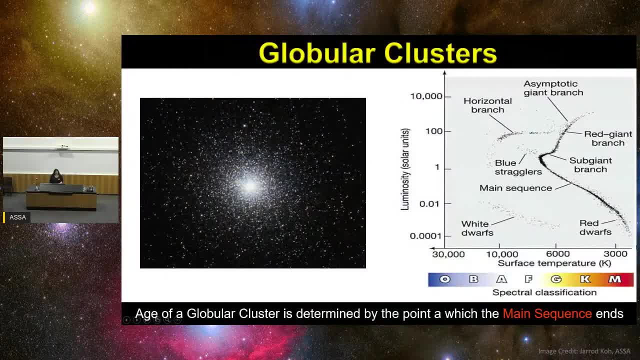 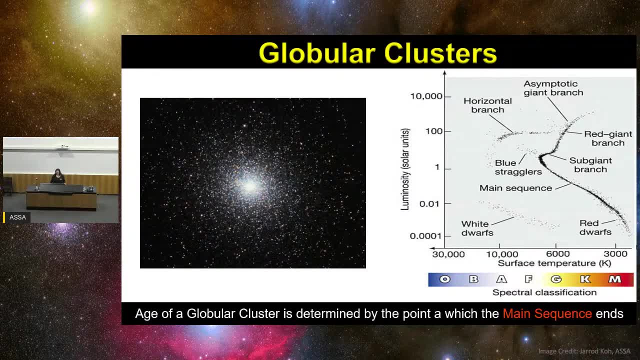 10., 10., 11., 11., 14., 14., 16., 15., 16., 17., 18., 19., 20. clusters, something like that orbiting our Milky Way: Beautiful objects to look at, But 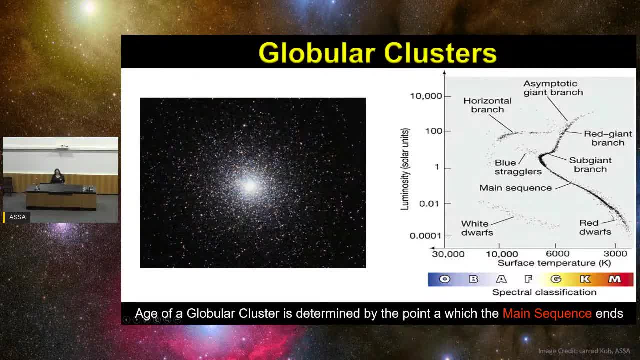 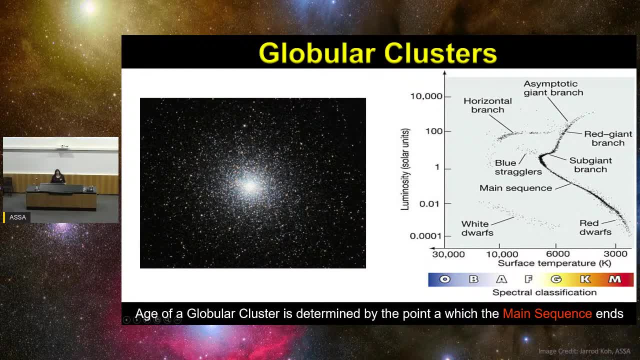 the HR diagram is actually used when they determine the age of these globular clusters. So the age of a globular cluster is determined by the point at which a main sequence star ends. So they find the main sequence stars within the globular clusters that they're. 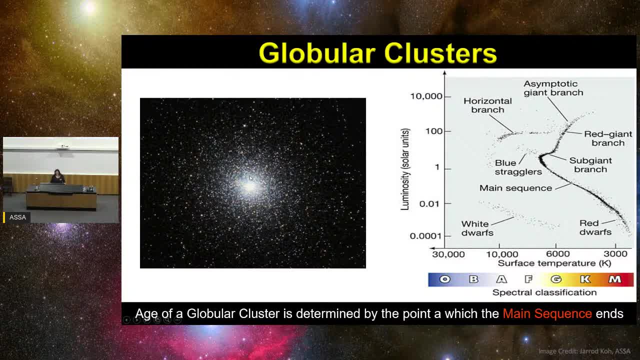 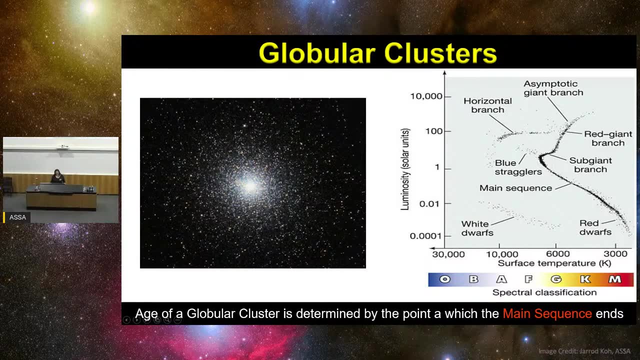 looking at This, looks like 47 Tuck. maybe it is. yeah, This is all Colin's presentations, by the way, And so they look for this. this is the knee that you were talking about, Colin, here. yep, So they look for this knee when stars start to turn and come off the main. 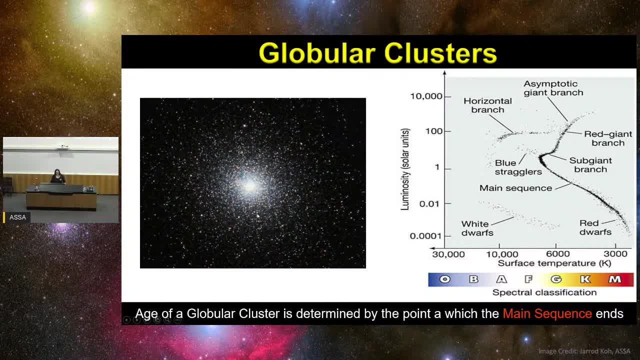 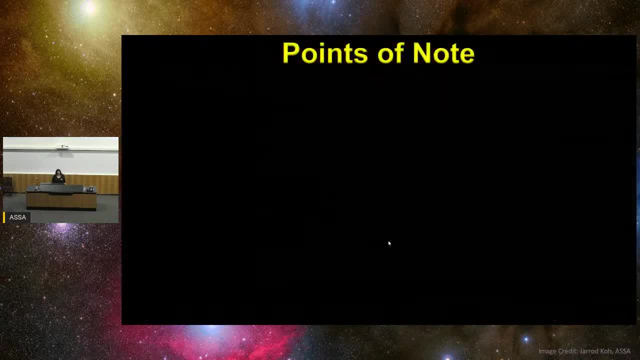 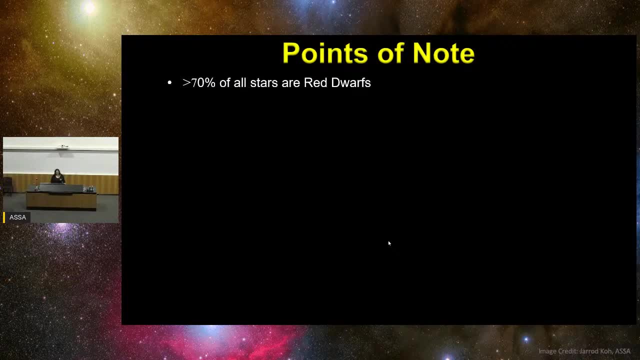 sequence and that's how they determine the age of the globular cluster that they're looking at. Okay, Points of note: More than 70% of all stars are red dwarfs. The stars spend 90% of their lives on the main sequence. Okay, So the biggest part, the main part of a star's life is burning. 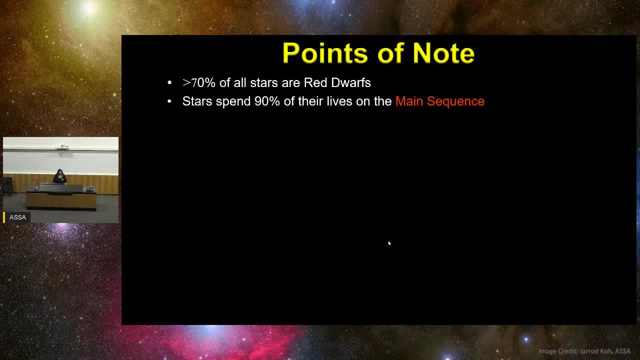 its hydrogen into helium. Main sequence: stars are burning only hydrogen, That's all. main sequence means They are burning their first stages through their first stage, Hydrogen, into helium. Again, it doesn't matter what colour they are or how big they are, If it's a main sequence. 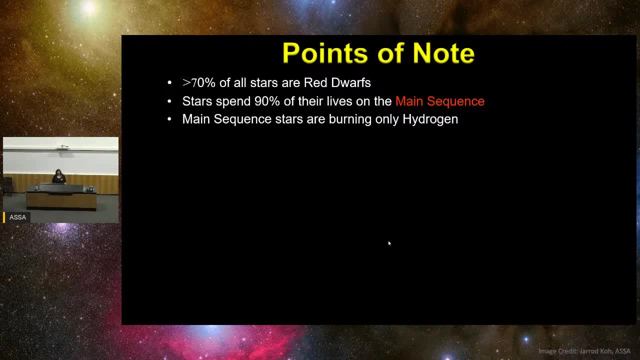 star. it is burning its hydrogen fuel into helium. Main sequence. stars are collectively called dwarfs. Again, that's just what they're called because they're on that first stage. It has nothing to do with their size. Giant stars fuse elements much heavier than hydrogen. 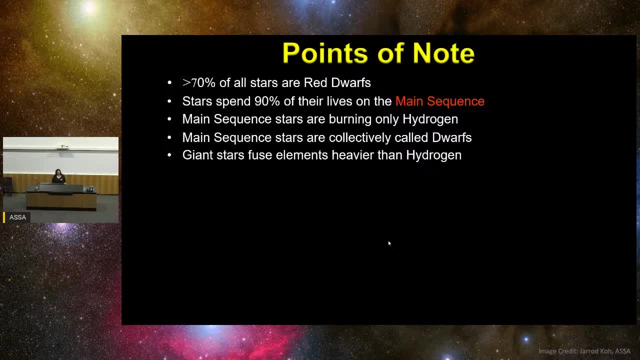 Okay, So they're burning their first stages. through their first stage, Hydrogen, into helium, And then they've got their second stage. They're hot star, They're burning up the receipts. So they're our first stars. ỏ White dwarfs, they are the cores, the hot cores of dead stars, So stars like our sun. 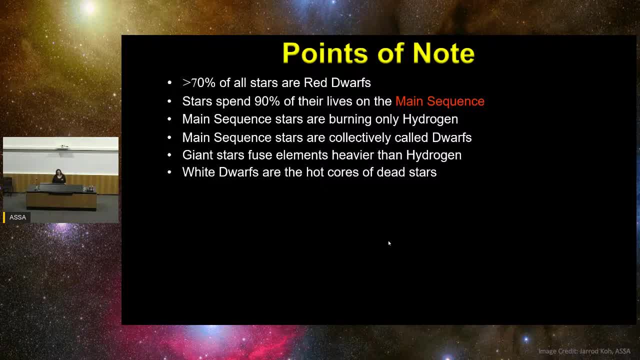 will end up as a white dwarf And a white dwarf- our core of our sun- will end up about the size of the Earth. That's quite remarkable when you think that you can fit, you know, 1.3 million Earths inside it right now. So the cores are actually going to shrink right. 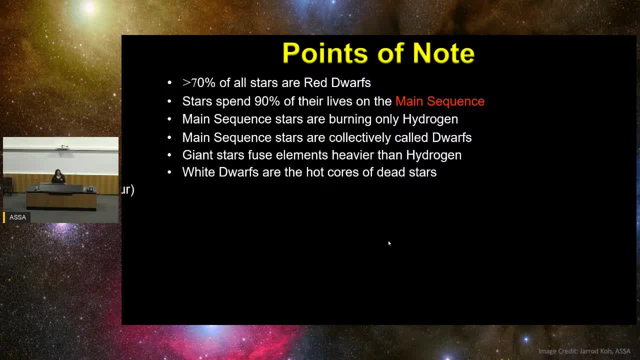 down And that's why they're very hot and very dense. Okay, So all these stars, they're called white dwarfs, which means they come directly. Brown dwarfs are called. they're failed stars. They're too small for fusion to occur. 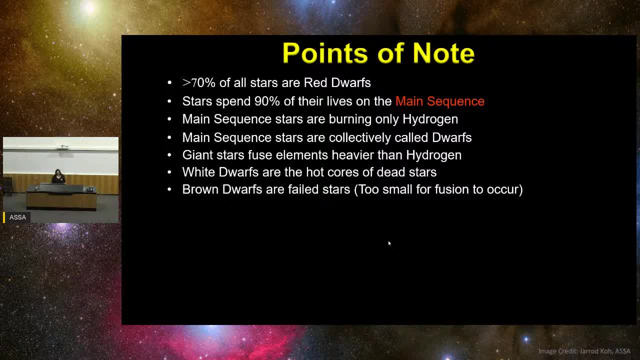 And brown dwarfs they are about. you need about 60 Jupiters, Is that right, Colin, In order for a brown to be a brown dwarf. So I've heard people say: is Jupiter a failed star? I get that question often. 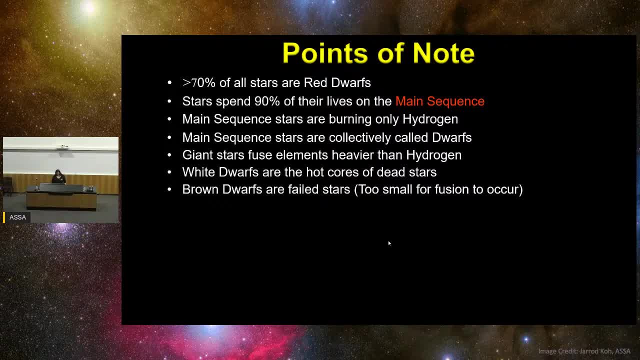 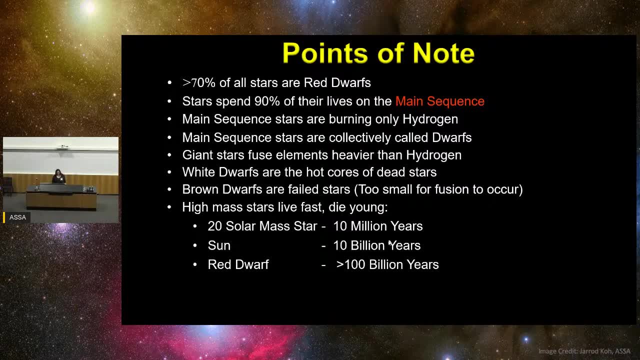 You need to be about 60 times the mass of Jupiter. Or brown dwarfs are about 60 times the mass of Jupiter, But high mass stars they live fast and they die young. So a star 20 solar masses might live for about 10 million years. Our sun will go for 10 billion years And a red dwarf over 100 billion years, And so the universe isn't old enough. We haven't seen one even begin to die yet, And class L is a mixture of red and brown dwarfs. 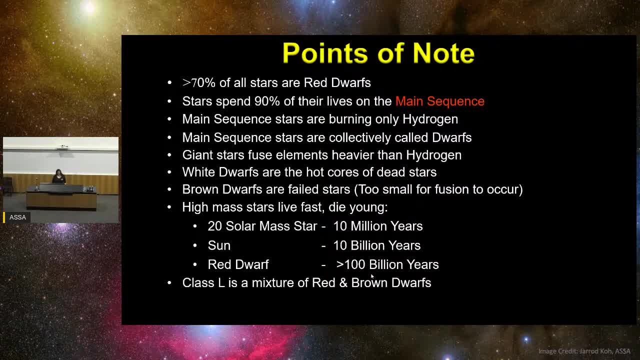 So there is another one after the M. There is a class L of red and brown, So that's been added on, And class T and Y are all brown dwarfs radiating mainly in the infrared, So not optical stars, not things that we can see through telescopes. 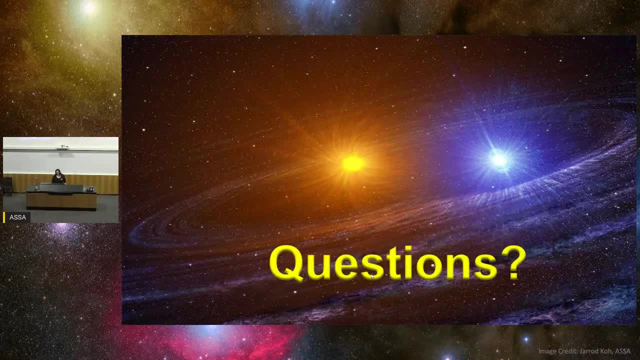 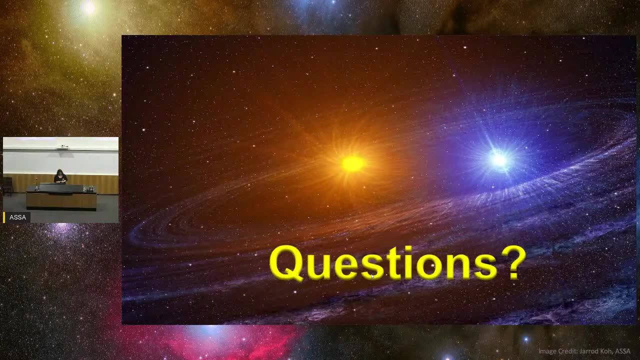 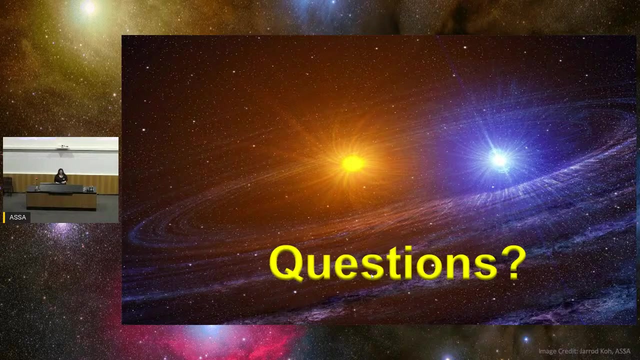 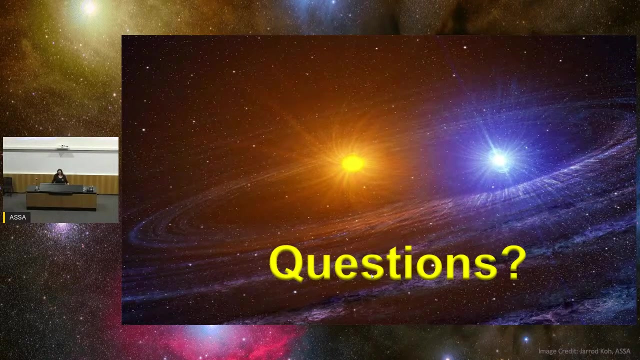 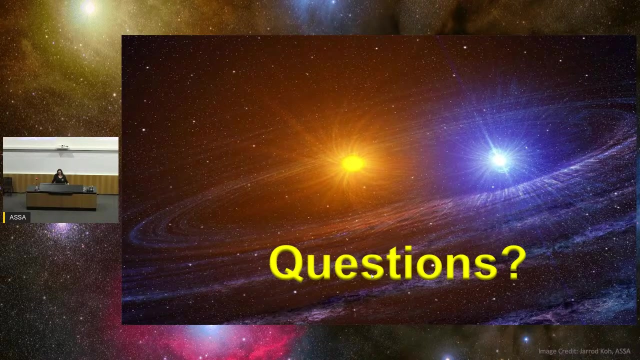 Questions. Do we have any questions In the audience? No, Are you all still awake? Yes, we have a question. Is Betelgeuse a red dwarf? It's a red supergiant. What's the difference? A red supergiant? 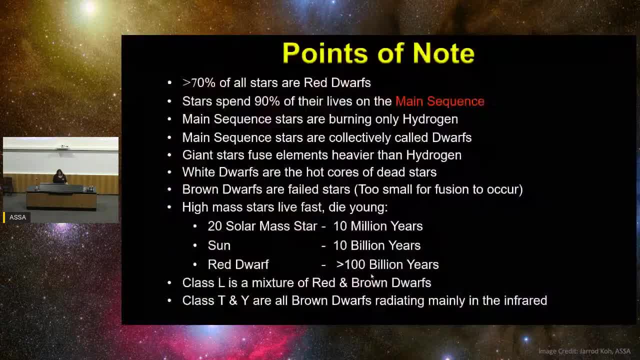 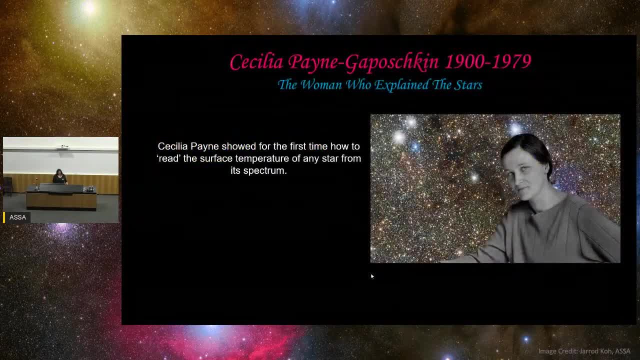 So a dwarf star, A star If I go back to? Sorry, Just give me a moment, I'll go back to my. It would be easier if I did it the other way. Hang on a minute, Here we go. Let's leave this up. 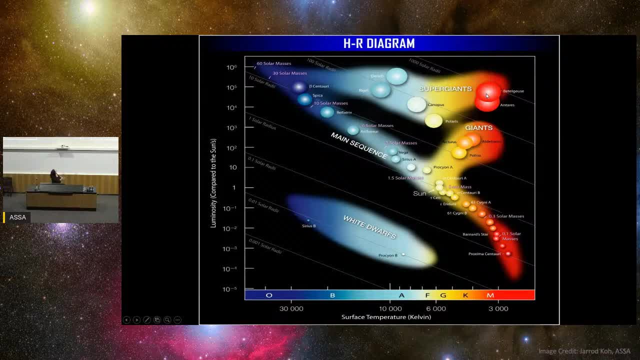 Betelgeuse is over here, I'll use. Can you see that one there? So Betelgeuse has come off. It sat around here when it was on the main sequence, So when it was burning it's higher, So it's moved from hydrogen to helium. 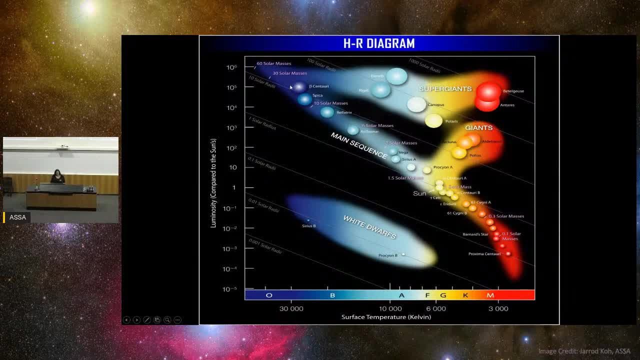 it sat on this part of the main sequence. up here Betelgeuse actually sits around. It's been between 11 to 20 solar masses, So it would have sat around here It would have been quite blue. But Betelgeuse is actually burning much heavier elements. 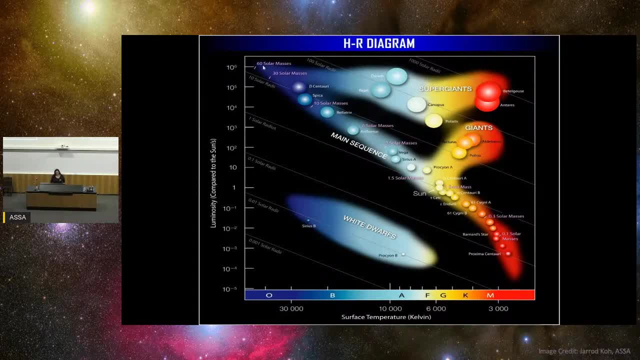 It's even gone past its helium burning stages, So it's burning much, much heavier elements. So it's moved off. Now stars up here will move off into becoming stars. So it's moved off Now. stars up here will move off into becoming stars. 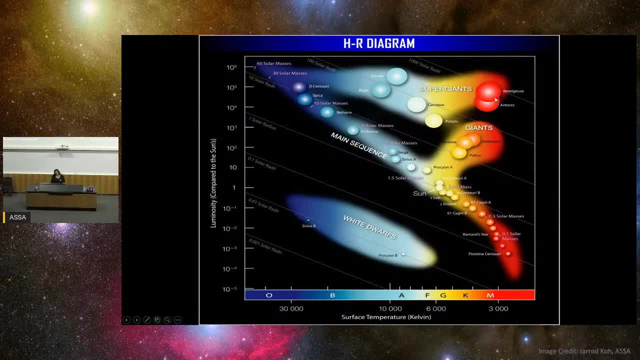 So it will become what we call a red supergiant. So your dwarf, I mean. we classify all of these as dwarf stars, But it's no longer on the main sequence, It's over here. Red dwarfs are over here. 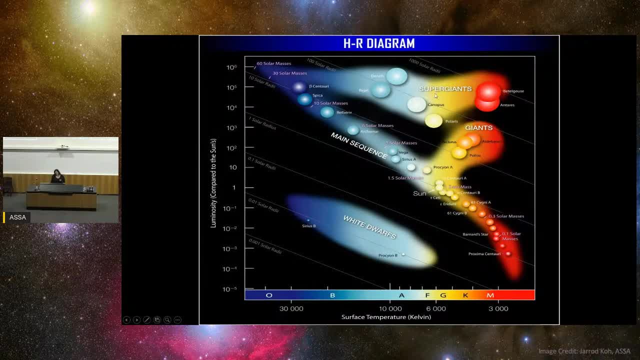 Sorry, the red dwarfs are down here. Red giants will be over here. Betelgeuse is a red supergiant. If you could swap. I mean, I know when I said: dwarf stars down here have nothing to do with size. 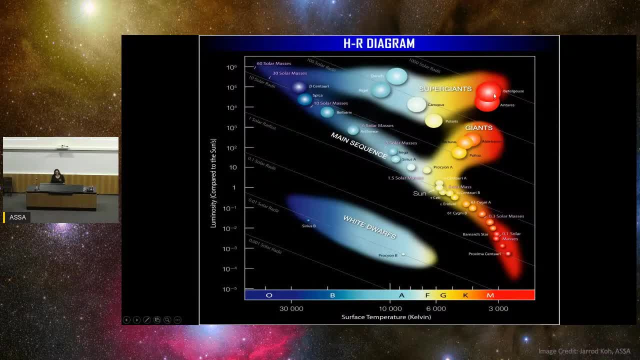 But it's moved off the main sequence. If you could swap Betelgeuse for our Sun, it would come out past the orbit of Jupiter. If you could swap Betelgeuse for our Sun, it would come out past the orbit of Jupiter. 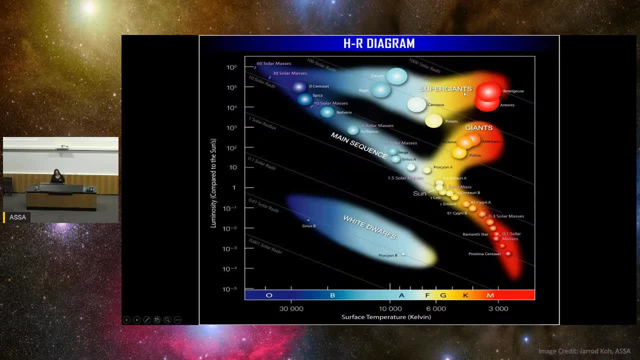 So it's no longer burning hydrogen to helium, It's burning much, much heavier elements And the star has become very small and very big due to that really, really heavy core. We think actually the core of Betelgeuse is over a billion degrees. We think. actually, the core of Betelgeuse is over a billion degrees. So they get very hot and the star swells right out. So they get very hot and the star swells right out. So that's the difference. here It's not a dwarf star. 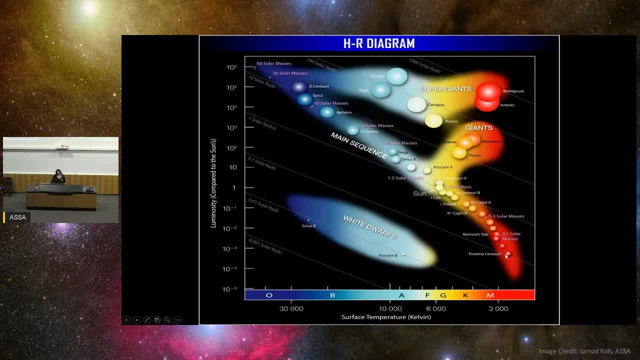 We could call them dwarf stars if they're on the main sequence. We could call them dwarf stars if they're on the main sequence. Red dwarfs are down here. White dwarfs are here. This is a red supergiant. Does that make sense? 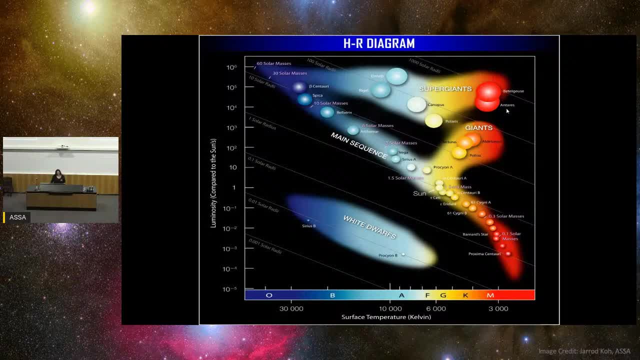 Does that answer your question? Is it still there? Is Betelgeuse, Yes, I mean. who doesn't look at Betelgeuse and think, just blow already. It's the shoulder of Orion, It's the red star when we look at Orion. 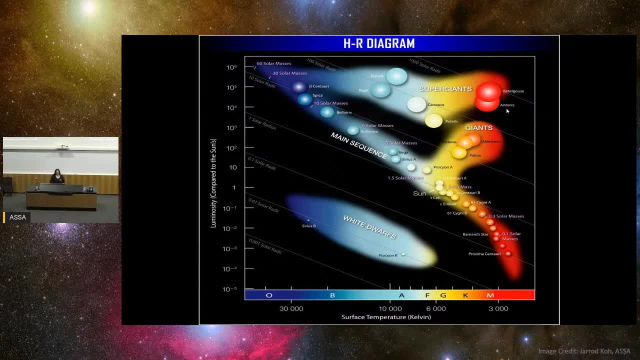 Remember, we see him upside down. So it's the red shoulder of that beautiful orange star in Orion. So it's the red shoulder of that beautiful orange star in Orion. So it is still there. But we need to also remember when we look at Orion. 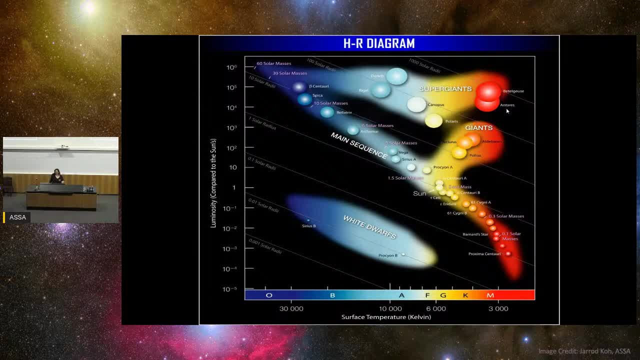 when we're looking at Betelgeuse, we're looking at that star as it was about 550 years ago, because it's 550 light years around, 550 light years away. So it may have already exploded, but we just haven't seen it yet. 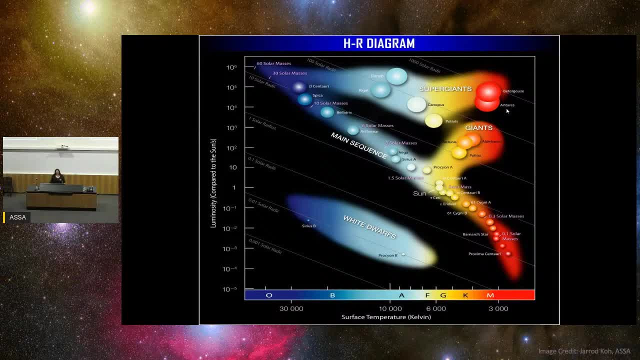 It would be something, though, to see that one go. My bet's still on Eta Carina. Oh, Eta Carina would be spectacular. Yes, I'll take the two of them in my lifetime. That'll be good. Any other questions? 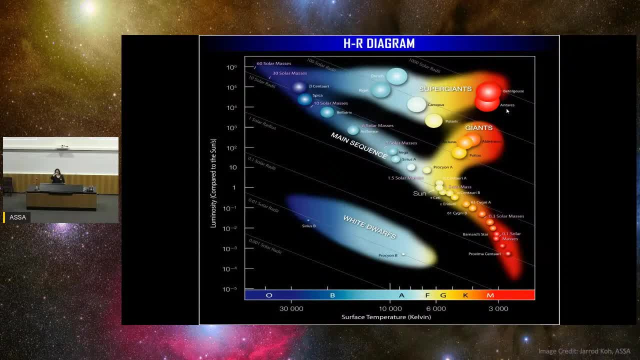 Behind you, Scott. Yeah, just an online question first. Dean asks: would we estimate Betelgeuse to be about 10 million years old? Would we estimate Betelgeuse to be about 10 million years old, Or I think you just answered that one before. 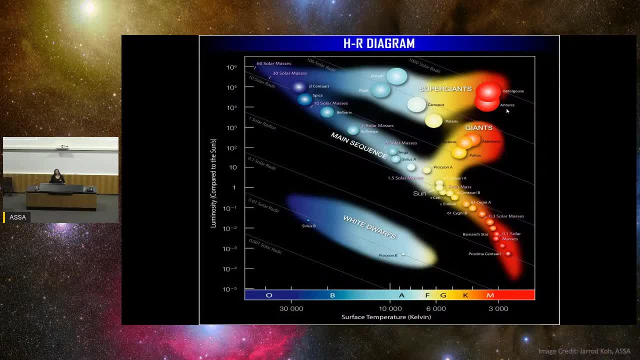 Or I think you just answered that one before. How old is Betelgeuse, Colin? It would be around about 7, 8 million years old. It would be around about 7, 8 million years old. We know with the elements. 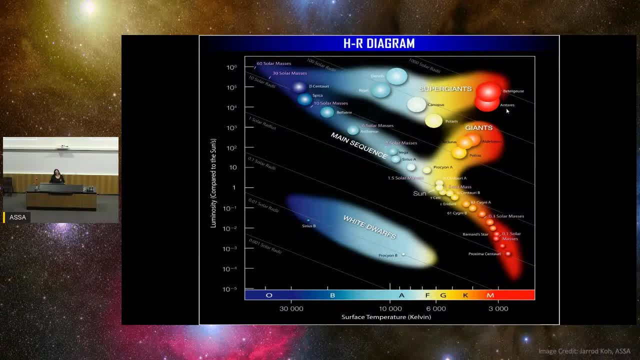 that it's fusing. at the moment it's around the neon stage, Am I right? The neon oxygen burn stage? So it'd be well over halfway. Yeah, Hi, So all the stars which are on the main sequence. if they are burning hydrogen, why is there such a difference in temperature? Because of the size? 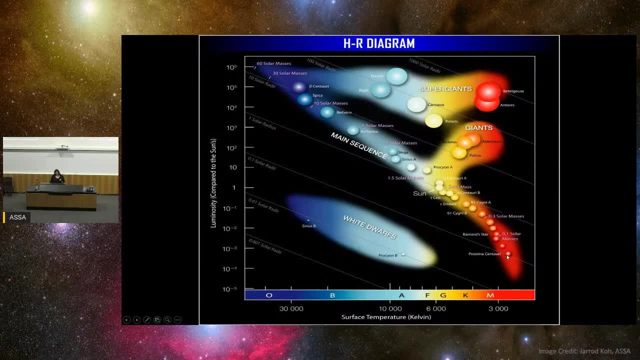 of the star. Okay, So, Proxima Centauri, this is that direct relationship that you see. We see it here. Proxima Centauri, you know about one-tenth the mass of the sun. It's not as big as our sun. 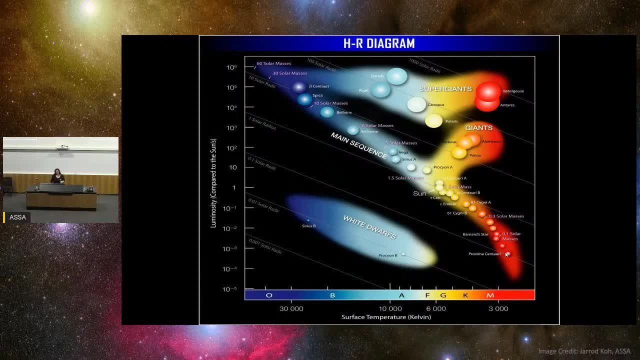 It's not as massive. So the more massive a star is, the hotter its surface is going to be. while it's on the main sequence, Okay. While they are fusing hydrogen into helium, Okay, It's something that one solar mass like our star will have a core temperature. 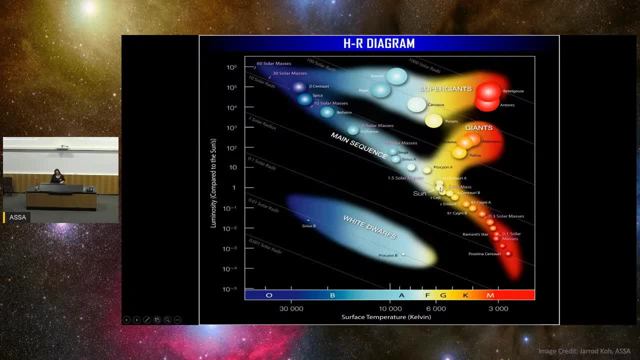 a temperature on its surface around 5,700.. These stars here, Spica and Hadar, these are a lot more massive than our sun. They're much, much, not just massive, but bigger stars, So they do have hotter surfaces. So that's the relationship. It is a direct relationship between the size of a 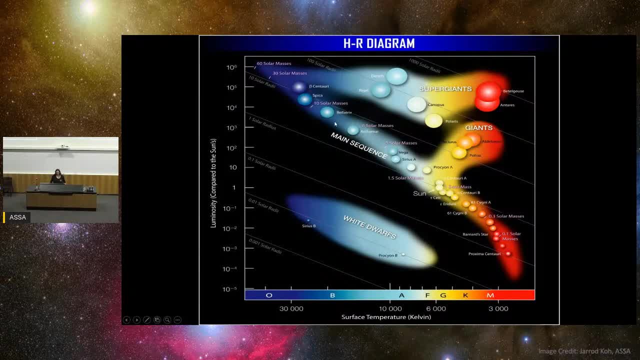 star and its surface temperature. The mass of a star, I should say, and its surface temperature. These also they burn their fuel differently. through a convection method, They have a different burning. The way they burn their fuel is a lot more different to what we have like, for example. 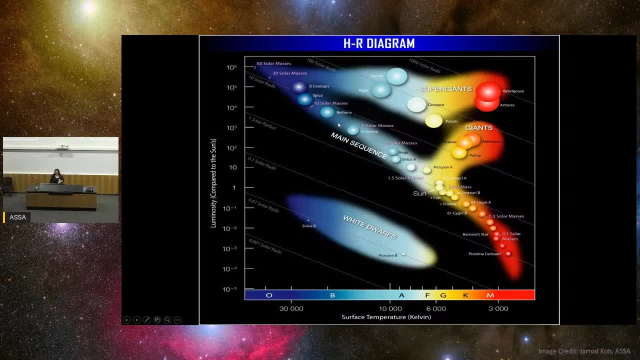 stars in our sun and stars much bigger. That one we go into in the next one, don't we Colin? That's in the burning, how stars burn their fuels, That's in the next talk. So do the stars go up Like? do they keep getting bigger? 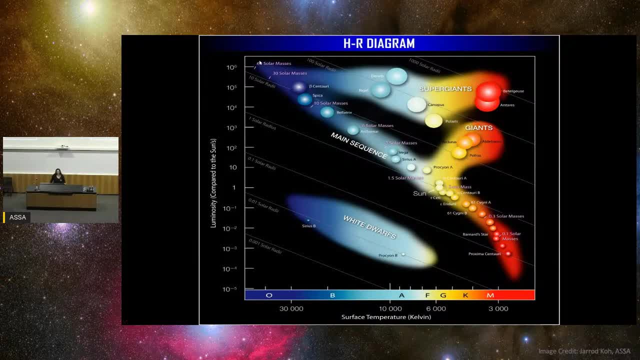 Oh, yes, We've seen. so. Eta Carina now, we think, estimates about 100 solar masses And there's a star- the most massive we've seen is R136A1 in the large Magellanic cloud, the most massive star, about 300 plus solar masses. So yes, they certainly can keep going. 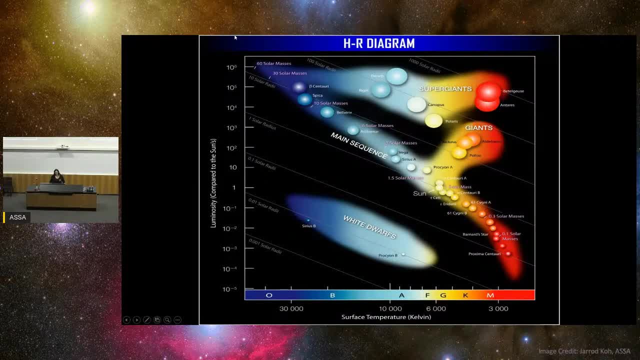 up this way And as they get more massive, they get hotter their surfaces get much, much hotter. Their life cycle, their lifespan, sorry- also gets much, much shorter. Any other questions Ian Online asks: do we know why Betelgeuse is varying in brightness and luminosity? 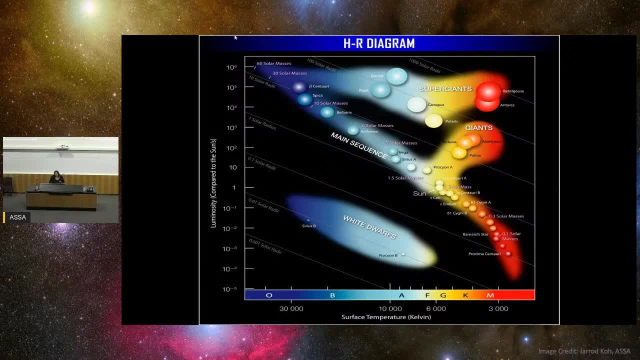 Do we know why? Why Betelgeuse is varying in luminosity, Why it varies in luminosity? Now it did dim. I think it started a couple of years ago where it started to dim. Yeah, that was scary. And then it brightened back up again. Now I know there was a dust cloud involved. I 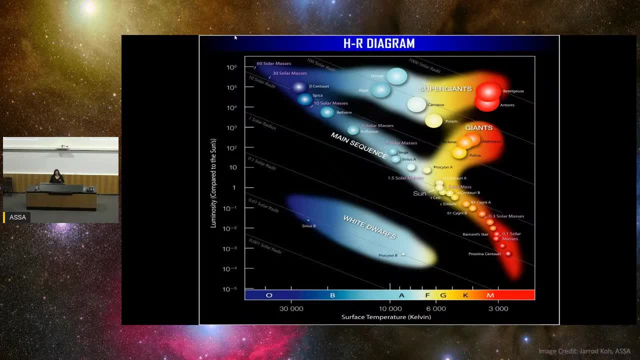 don't know if it's throwing off Colin, is it throwing off parts of itself? And there's a dust. it moved through a dust, a bit of dust, where it started to dim it. It is, It is, And that's again because it's at the end of its life. It's getting they become. 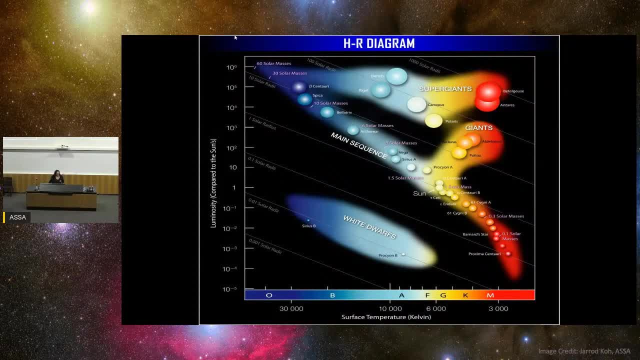 unstable. It's like almost: Hey, Almost, Almost, Almost, A little more Almost there Again, we'll go into that one, next, next with the next talk. But yeah, so there was dust involved, So it passed off. I think it actually because they have. 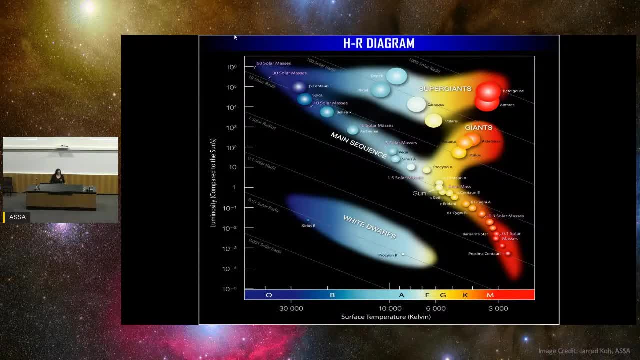 very strong winds, these stars like Betelgeuse and Antares, So I think it threw off quite a bit of itself And the dust around it actually is a bit of dust. Yeah, dimmed its brightness, yep. 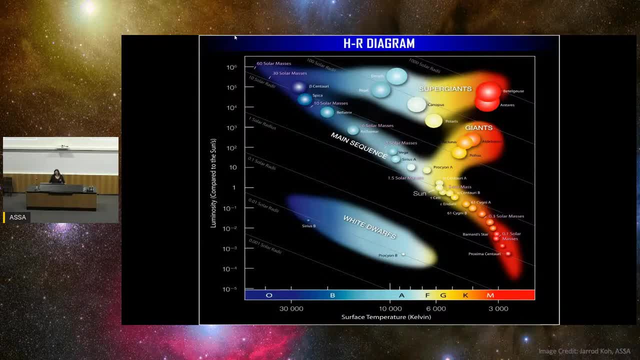 But it got really dim. Yeah, Do you remember seeing that? It got really really dim and it's brightened back up again. Now it's dimming again, I think now. So it does this, but, as Colin said, it is a variable star as well. 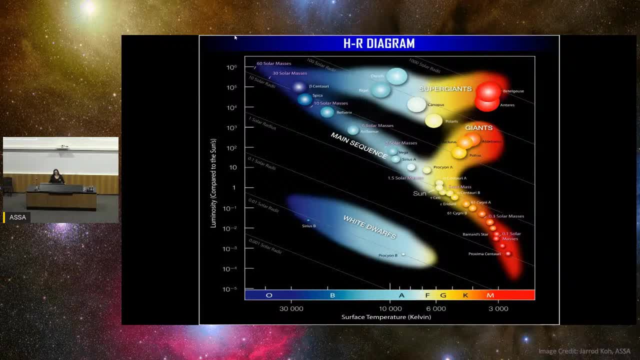 I think we're all in. Anyone else, Any other questions? Comments? Anyone want to add anything more? Colin, do you want to add anything? Oh okay, Adi, did you want to add anything? Yes, this young lady over here. 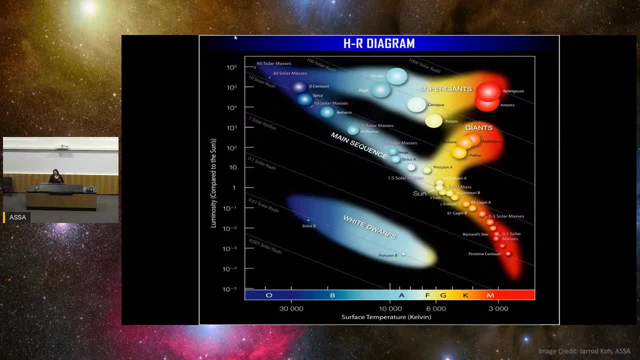 Just put your hand up, Ryan. Thank you, Thank you. So how do you know how long the stars will live? I mean, like the predictions. how do you make that? Again with spectroscopy, when they look at the emission lines? 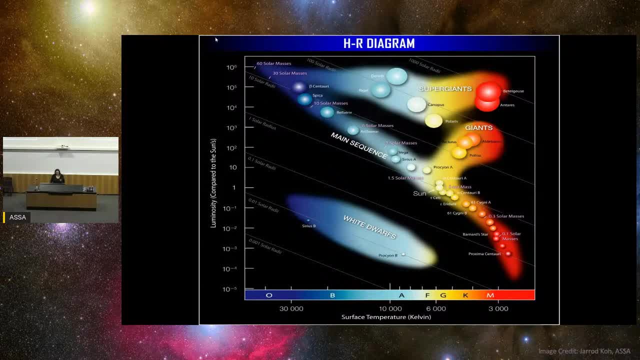 they can pretty much tell what a star is giving off Also by its temperature and its mass. So you look at a star that has a certain mass, that is red. you know it's covered with. He's doing that. He doesn't like me tonight. 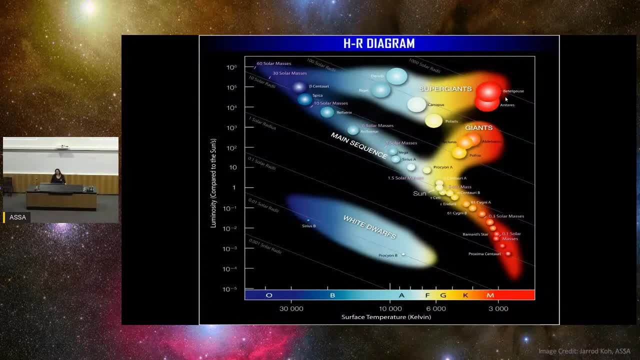 Yeah. so with stars like Betelgeuse, again, they look at the emission spectra, the absorption spectra- sorry, coming off that particular star as well- And by the temperature that it would be at, as to what elements is actually burning in its core at the moment. 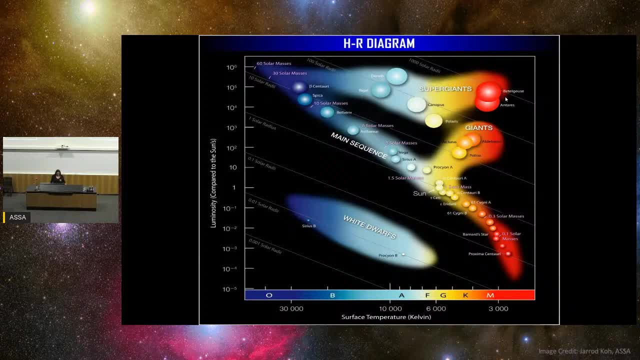 So I think Betelgeuse is at its neon. I remember reading in the last report: it's at a neon 80, would you, Could you help me out here With Betelgeuse? what phase is it in? Is it a neon? 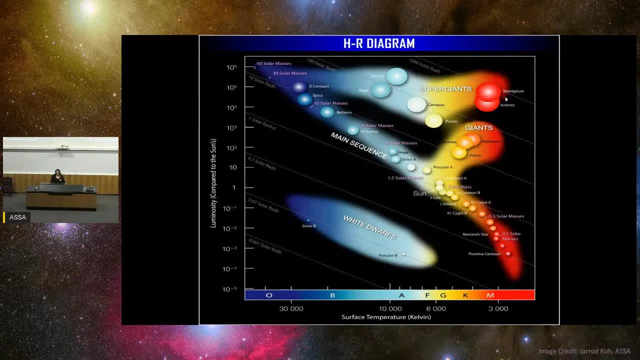 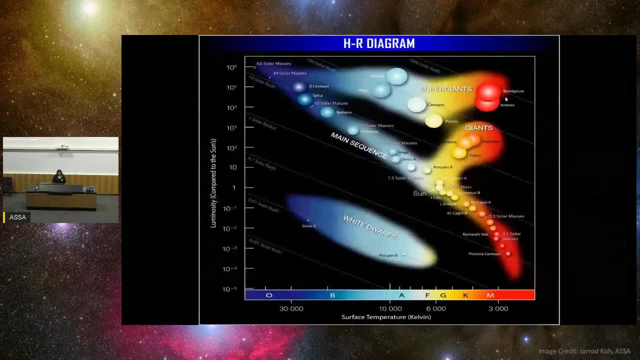 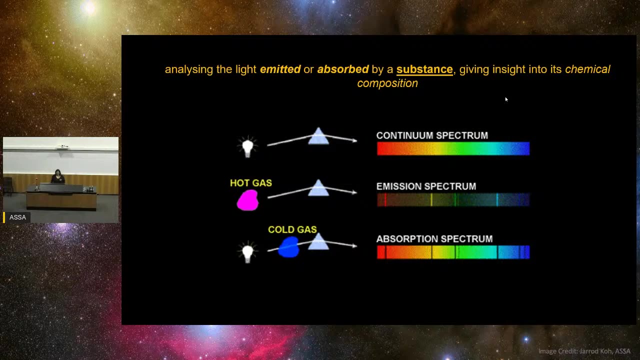 Okay, Yeah, it's near the end, So this is what they look for. So if I go back to Hang on a minute, Sorry, Probably Here we go. I can tell what emission, what elements, the star is made up of. 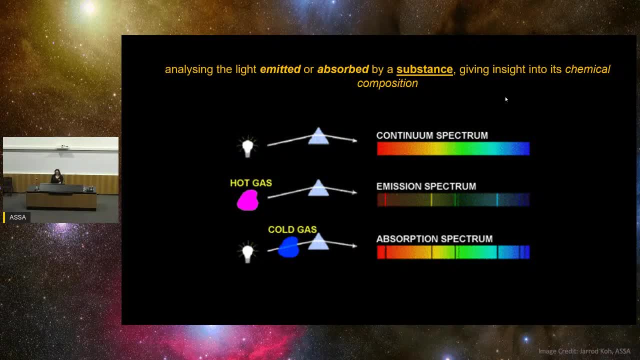 and what it's actually fusing. This is what astrophysicists do. when they split light like this coming looking off certain stars, or if they're looking from certain nebula, they can tell what it's made up of. 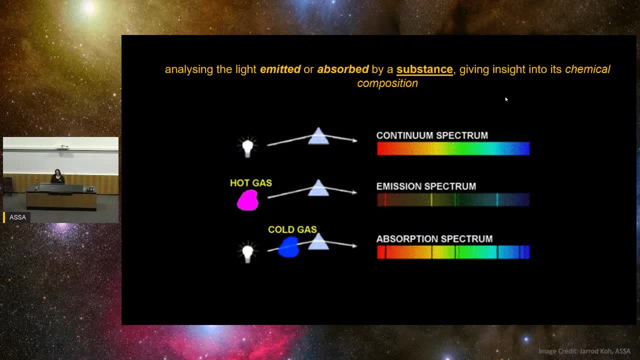 And again, the colour, the surface temperature of a star tells us a lot as well about where it is in its evolution. Yep, Thank you, Thank you. Do all stars at the end of their life? do they explode and create a supernova, kind of thing? 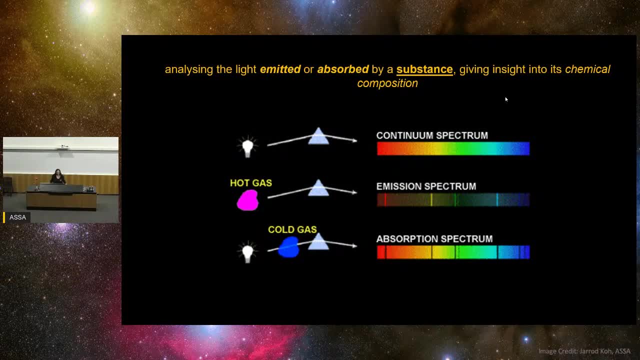 No. So very big, massive stars, So a star, for example, the size of our sun. no, it won't. It doesn't have enough mass, It won't go past that carbon and oxygen burning phase. It doesn't have enough mass to sustain a core at 500 metres. 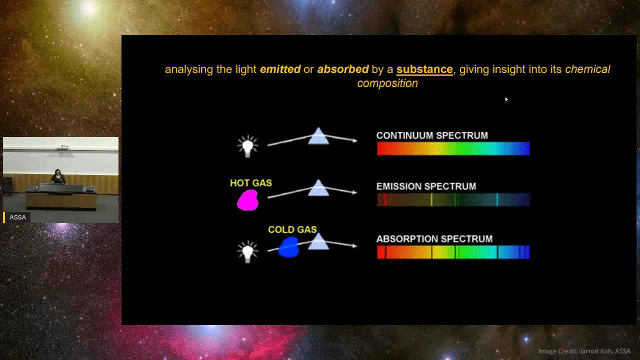 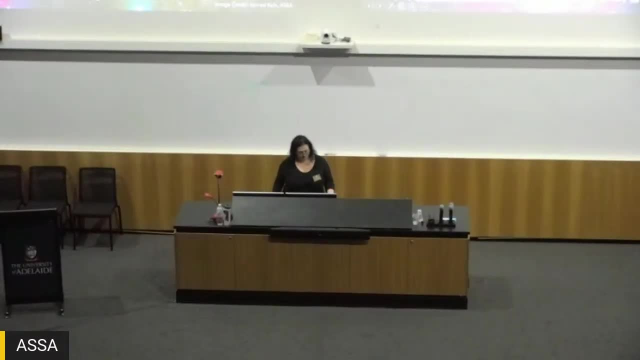 It doesn't have enough mass to go up to 100 million degrees and keep burning. There's not enough of it in its core. Massive stars, however. I'm just going to, If I escape this down. Ooh, What did I just do? 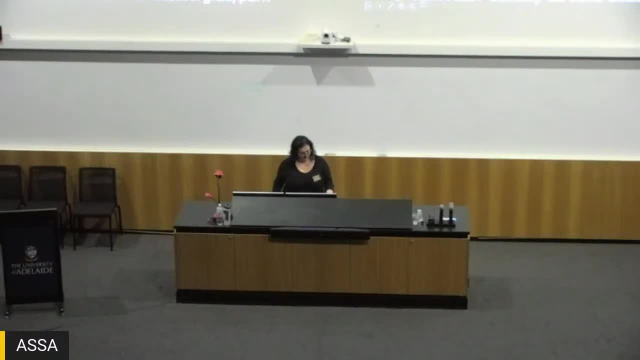 Hang on a minute, Scott. How do I get back into That doesn't work. Uh, I want to get back to my presentation. Sorry, I'm not a Windows user. Can you tell? What do I do Control? Oh, thank you. 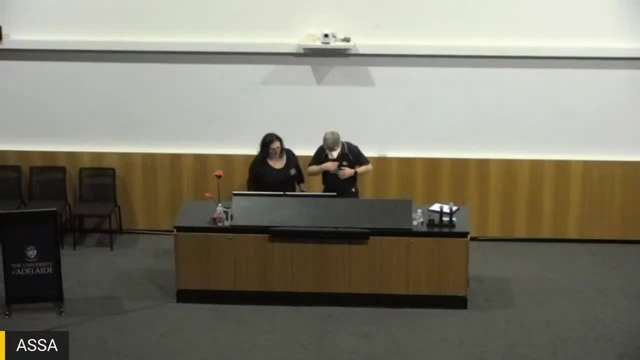 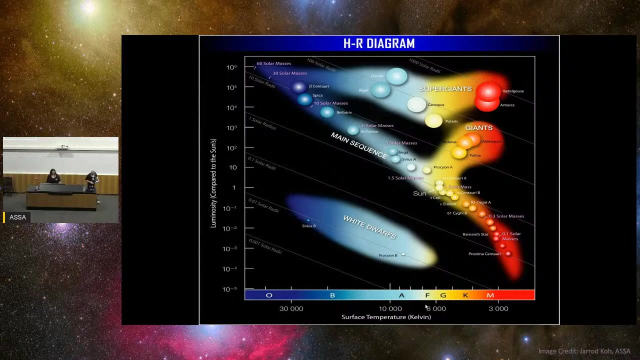 Thank you. Can I just make that bigger? That's Control and tab. Oh, is that what I press? Okay, Thank you. Thank you, Okay. so So your question: Sorry, do all stars explode as a supernova? 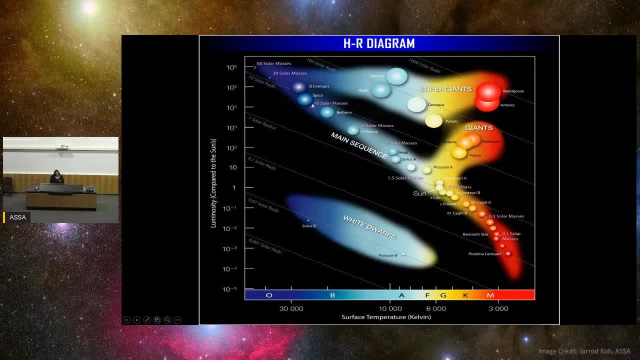 So stars pretty much turn solar masses upwards. We think they may explode as a supernova. They have to be up here. Stars like our sun, Sirius A, V, up to three solar masses Even, we think six to eight solar masses, probably not.